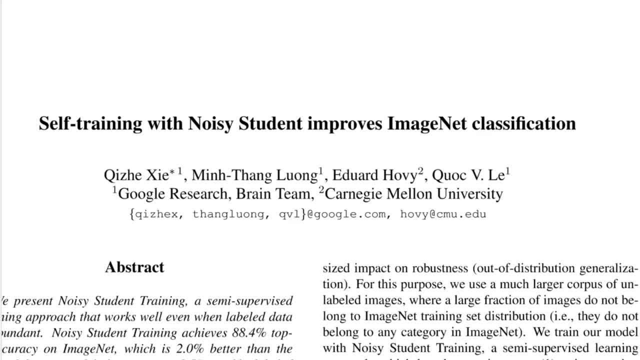 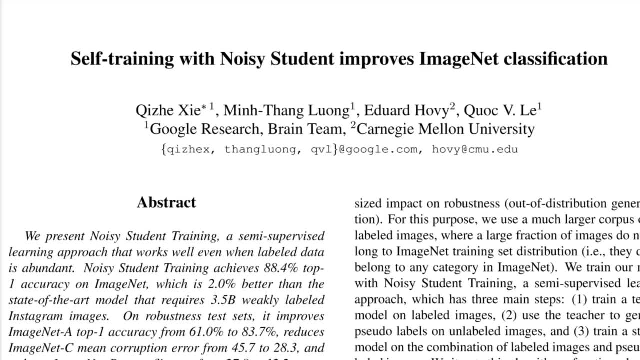 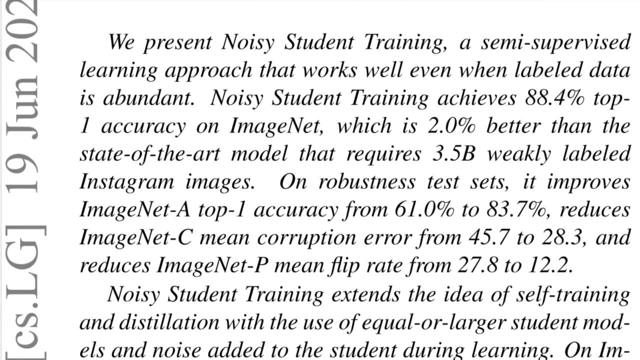 this all work, And today we're going to explore how this paper does it and what they say is important. If you enjoy content like this, as always, don't hesitate to share it out or tell your friends about it, And if you're not subscribed yet, then do so. I would appreciate that and you'll get more content. 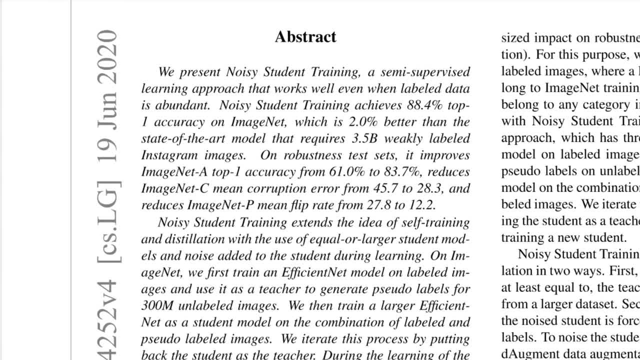 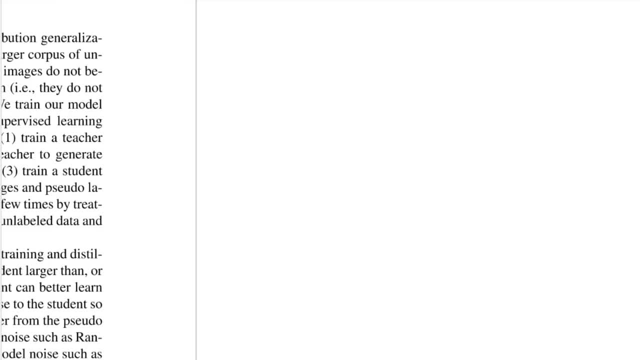 So win-win. So this paper is about semi-supervised learning in effect. So it's at the intersection actually of semi-supervised learning, knowledge distillation and transfer learning. So what do we mean by semi-supervised learning? Usually in supervised learning you'll have some sort of 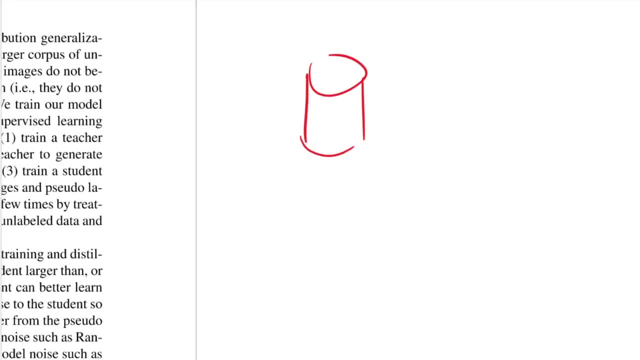 dataset, and the dataset will contain images. Let's say it's an image net, It's image dataset, So the dataset will contain images. This is an image with like some sort of cat on it and it will contain the labels according to that, So cat. 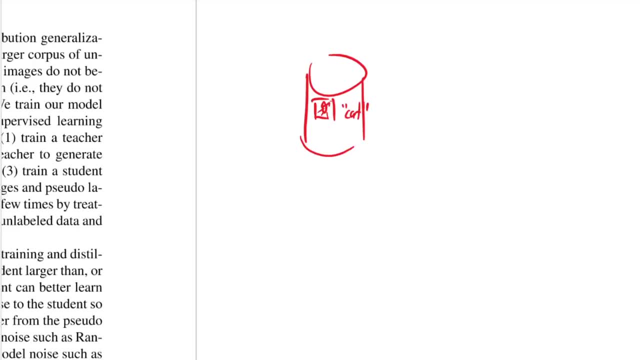 Now, in semi-supervised learning, you you assume that. so this is supervised learning. in semi-supervised learning, You will assume that only part of your dataset has the labels, so, like only this part down here, itthat can be identified as sub-supervised or Adobe, as usually it looks a little simplistic in an bake journal and 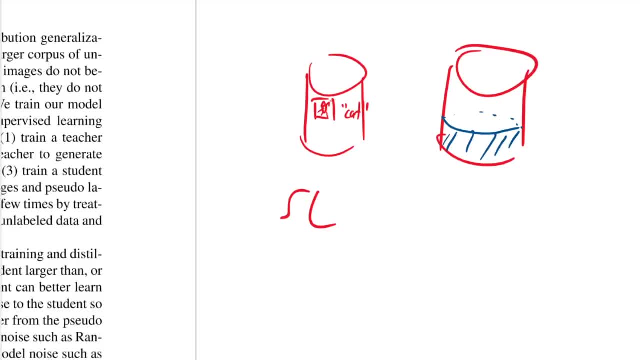 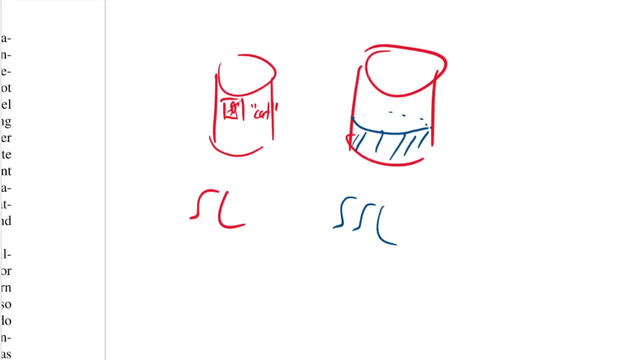 has the labels and the upper part does not have the labels. So that's semi supervised learning. It's often the case when it's very expensive to get labels So you can only get labels for a couple of images in your data set. But very often in semi supervised learning you still assume it's the. 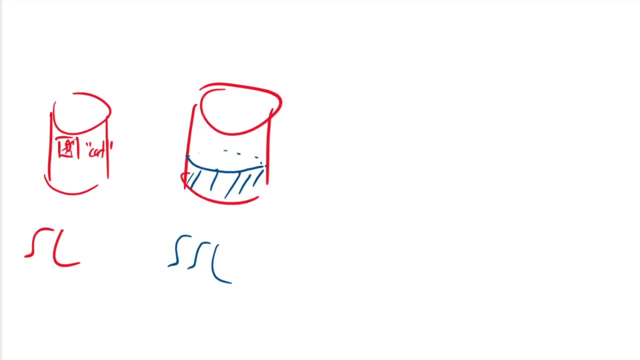 same data set. There is a slightly different setup here. that's called transfer learning. So in transfer learning what you'll have is you'll have your data set that has the labels, but it's very small. So you'll notice I've drawn it smaller. that means you have very little. 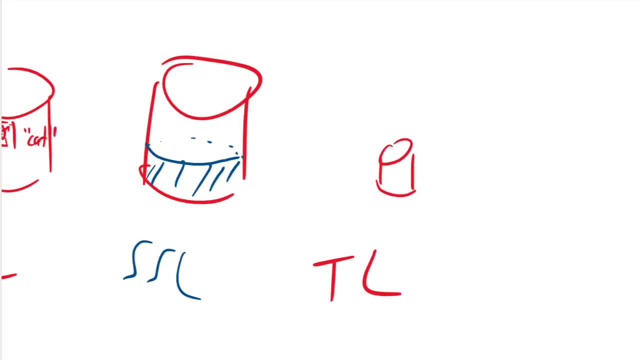 that is also the case when it's very expensive to get labels, but also it's expensive to get the data itself. This is often the case, let's say, in medical data, where not only is it expensive to get labels for, like, a CT scan, it's actually expensive to get the CT scan. So what the goal? 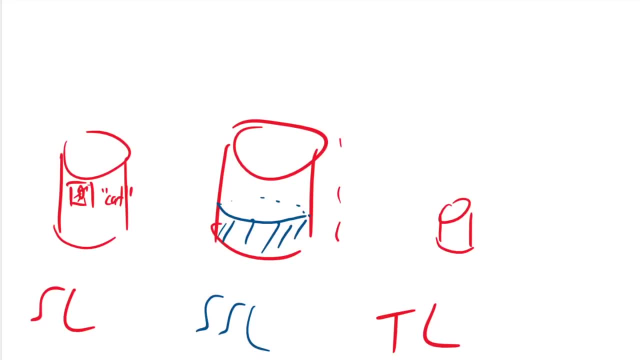 in transfer learning, is is to say, well, I do. I do have have only this small data set, but I do have this giant other data set over here. Now, can't I? it's not the same it's. maybe they're not CT. these are CT scans. maybe these are x rays. 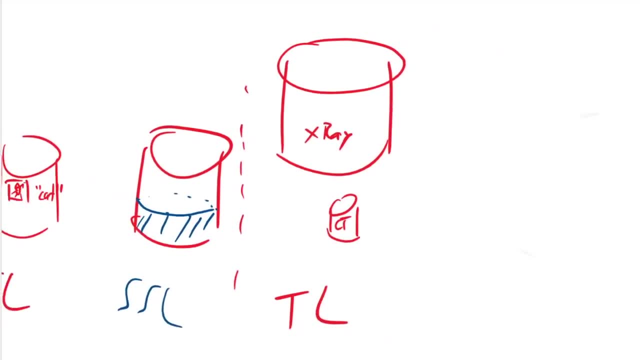 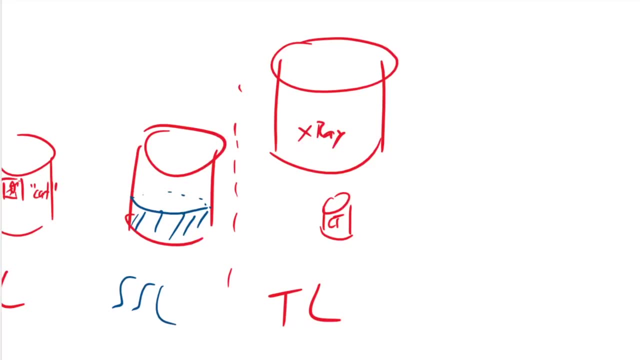 right, They're fairly similar, similar technology. If you slice the CT, it'll give you sort of an x ray. Can I, you know, train my model, pre train my model on x ray data and then fine tune it on? 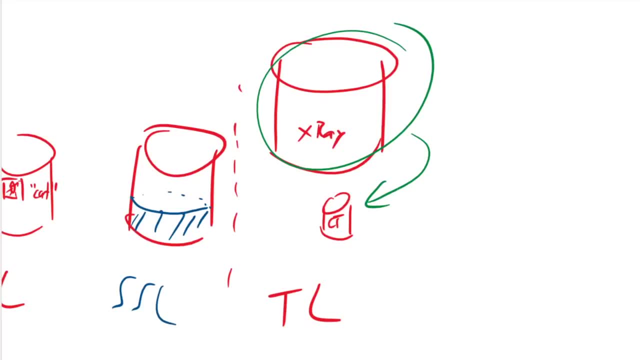 the CT data. So that's called transfer learning. usually, Now, this can be done with or without labels. So it can be that for the x ray data set you do have the labels or you don't have the labels. there are. 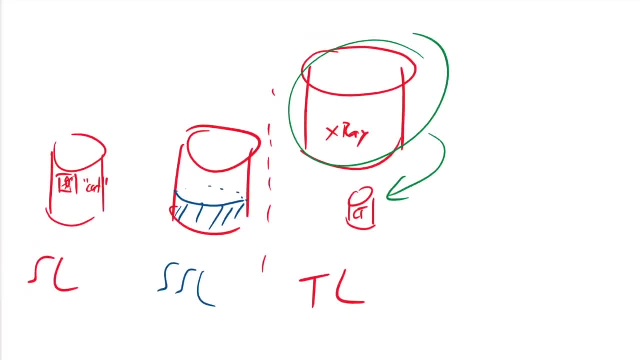 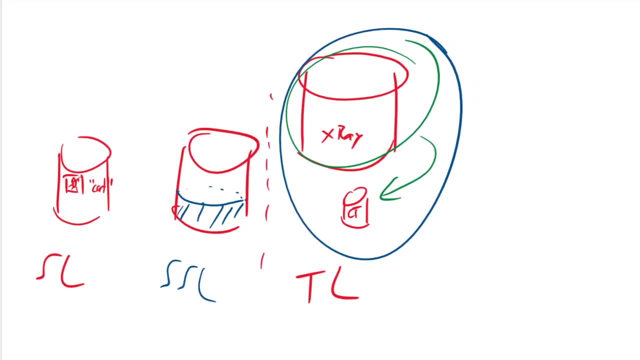 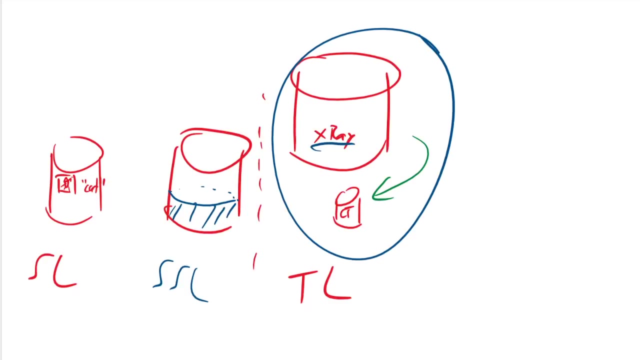 techniques for all of those. Now, what we're going to look at today is kind of the situation right here. it's the transfer learning situation- where you do not have the labels for this x ray data set, But other than in this x ray example, what we're going to look at is the small data set. 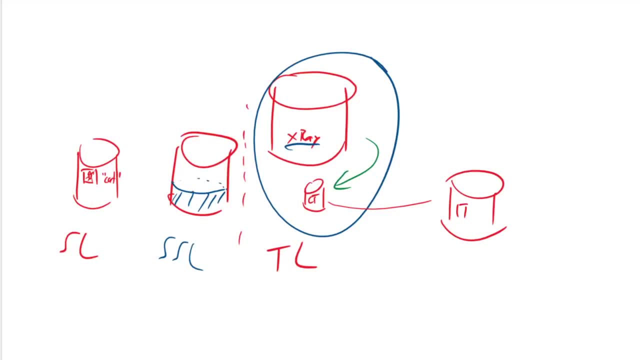 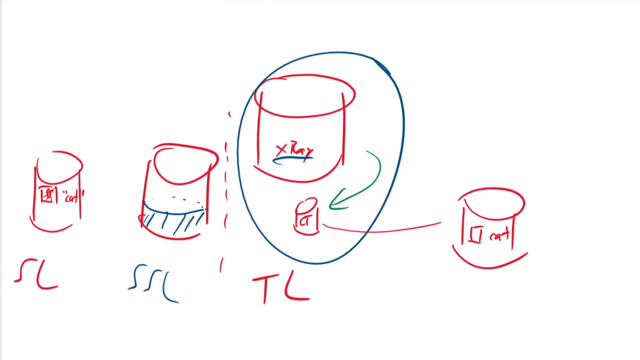 is going to be our image net database, So our original picture with label database. So you'll see immediately. the difference here is that in the transfer learning setting we usually assume that the data set we want to train on is fairly small. Here, you know, image net is already sizable. 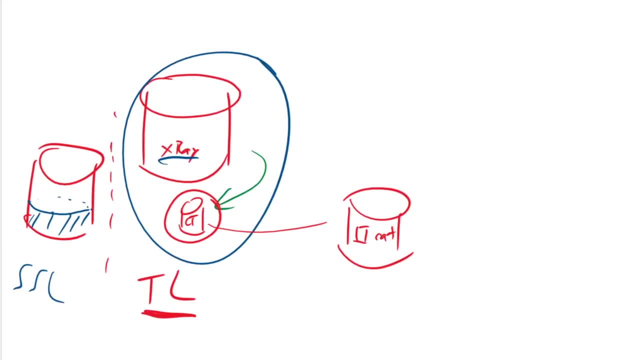 But what we have is we have a much larger database of unlabeled images that we can just get from the internet. So we can scrape the internet for any kind of pictures And that will be our unlabeled data set, And what we'll try to do is somehow incorporate this unlabeled data set here into 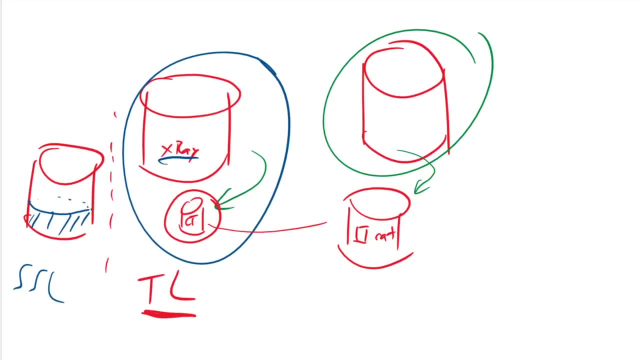 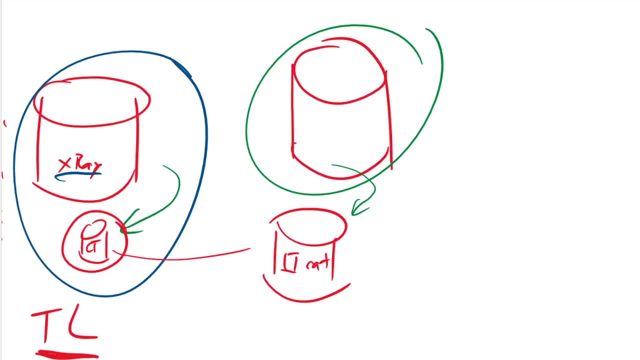 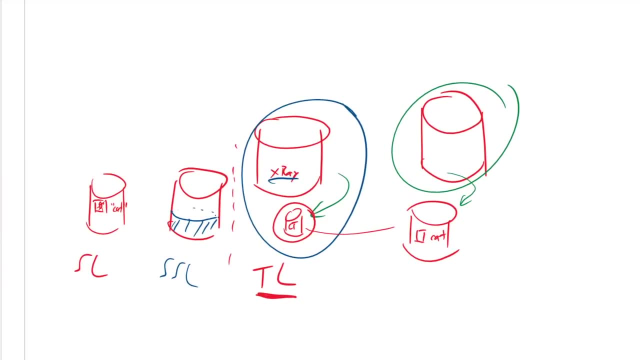 much larger data set of unlabeled images and you somehow want to make use of them. So I hope you see how this is sort of connected to the others. is it's essentially so sort of a transfer, semi supervised learning setting, But with the exception that usually in transfer learning 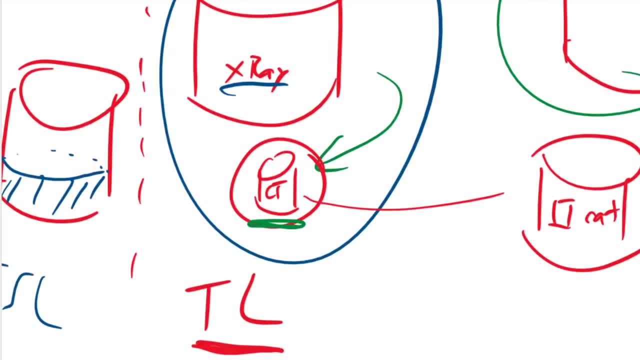 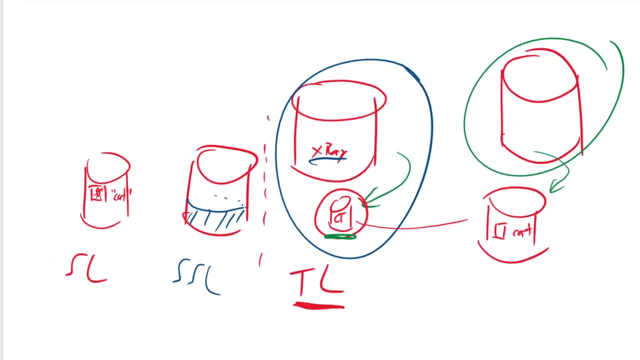 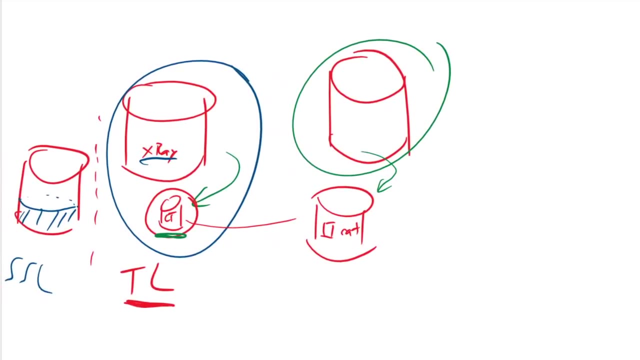 you assume that the, the labeled data set, is like super small, which is not the case here, And that's going to result in us being able to apply a different technique. So this different technique is called the noisy student. Now, usually what you might do in a transfer learning setting is you. 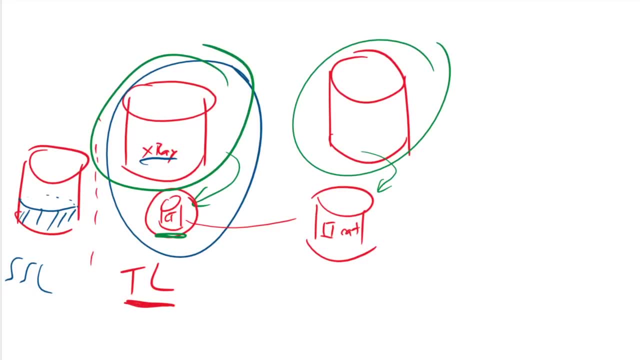 might want to start with that big data set, right, Because that's the data set that's sizable enough to allow you to train a really big model on it, And then you fine tune and you, you sort of hope that the information transfers over Here. on the other hand, what we want to do is we start with 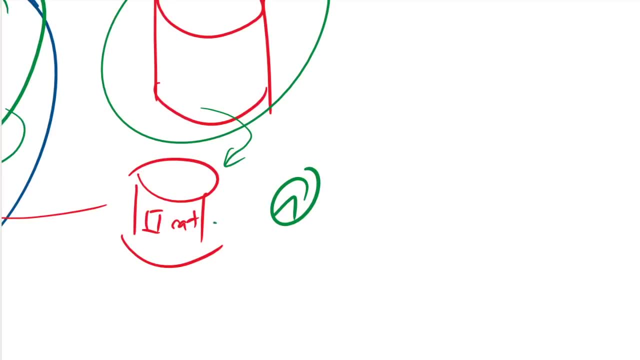 the image net data set. So first we train this in a supervised learning fashion into our model. Now this model is going to be called the teacher model. We know how to do this. we know how to train image net models right. So we can train this into a teacher model that has a 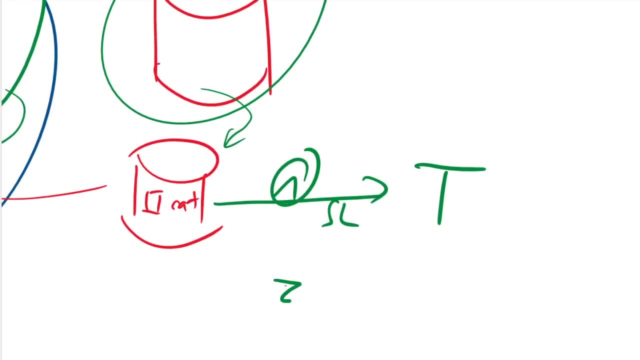 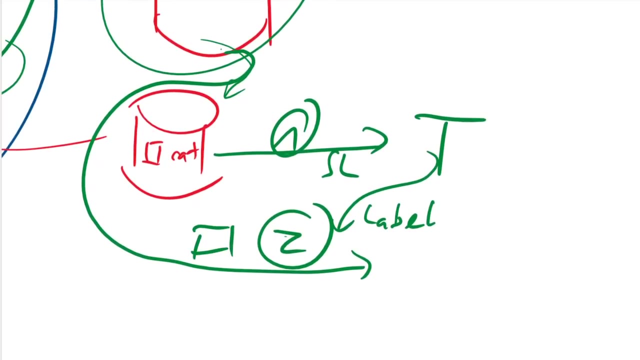 reasonable accuracy on the image net data set. Step two: we're going to take that big data set over here and use the teacher model to label the unlabeled images. So for each image, um, for each image coming in here, the teacher- so maybe this is again another cat. the teacher will say: that's a cat, Okay, so 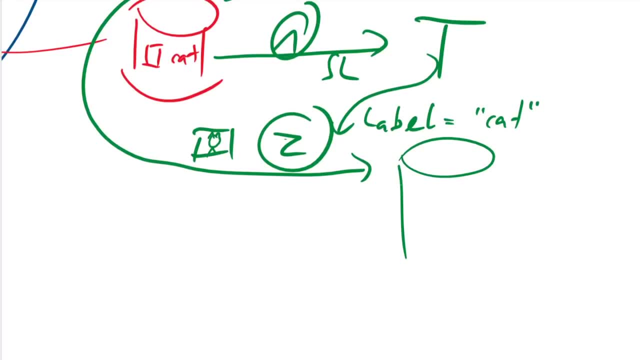 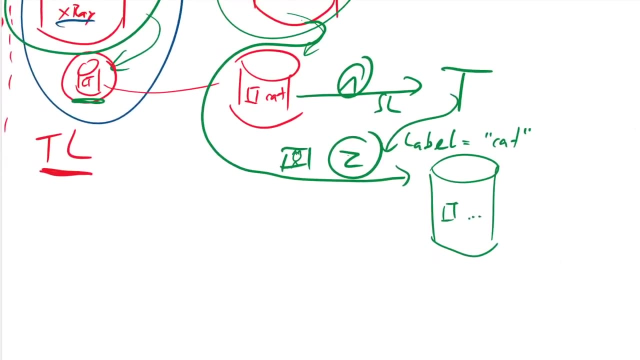 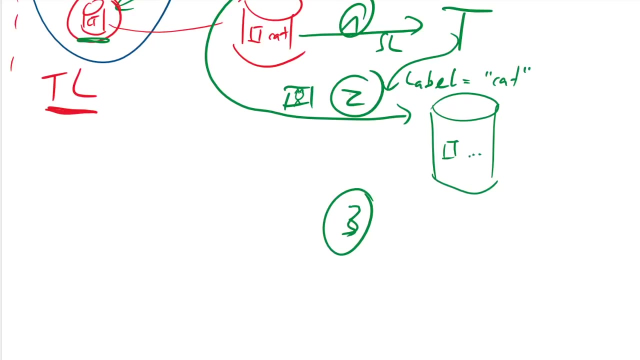 that gives you the big data set, where now you have images along with labels. just the labels aren't true labels, they're generated by the teacher. And then, in the third step, you train this big data set, you train on this big data set. 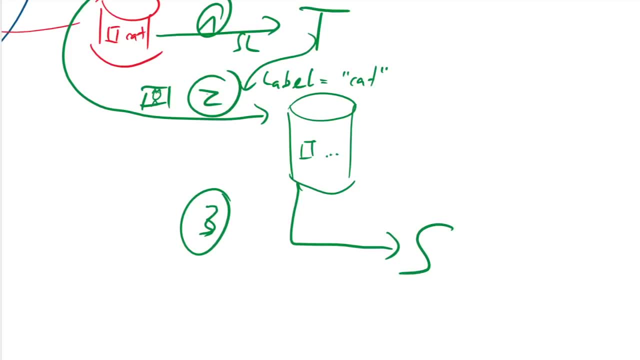 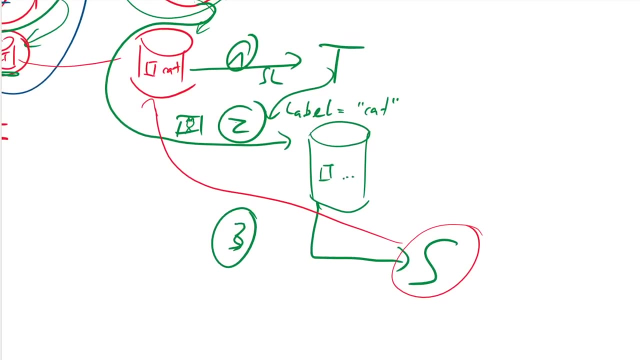 and that's what you call your student model, And then the student model. in this paper we'll see how can we make it such that the student is then better at the original image net task than the teacher ever was, which seems counterintuitive at first, because all of the information that the 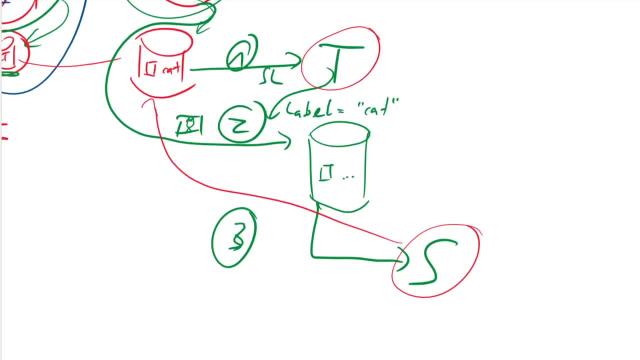 student is trained from is basically what the teacher already knows, right? all the labels here come from the teacher. therefore, the student shouldn't be able to outperform the teacher. But in this case, the student will be able to outperform the teacher, And their argument here is: 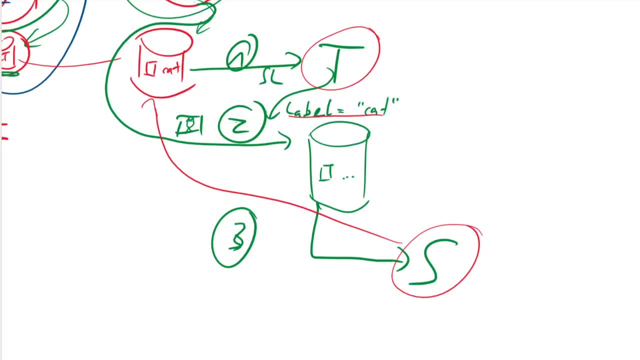 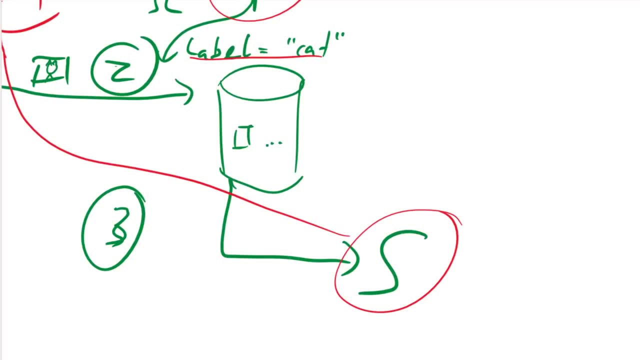 that this is mainly due to the fact that you use noise in this training procedure. So, when you train the student, what you'll do is you'll use noise, And one of the types of noise is that you severely augment this data right here in order to train the student. Now, we've known for a long time that data. 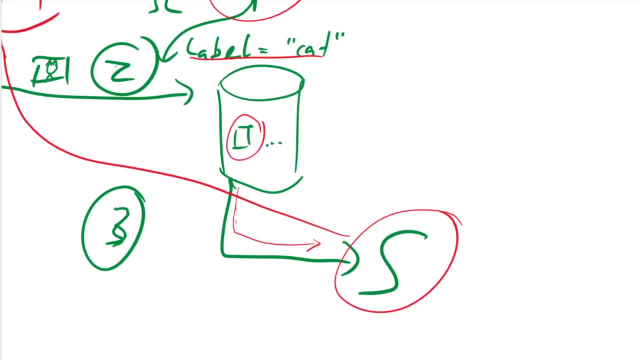 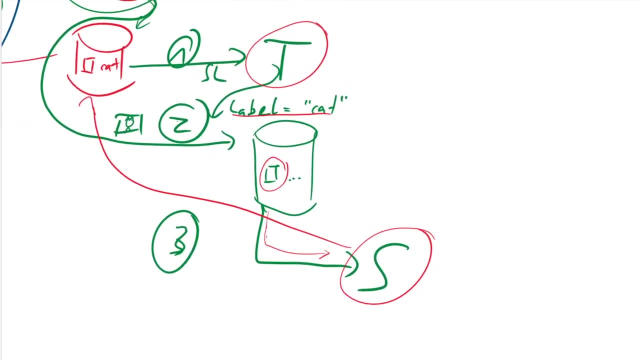 augmentation, for example in the frameworks of self supervised learning and so on, can have a very large benefit to training, And here the fact that we incorporate this, add extra data and we use noise and augmentations on it is going to result in a student that can sort of learn more about the data than than the teacher did. 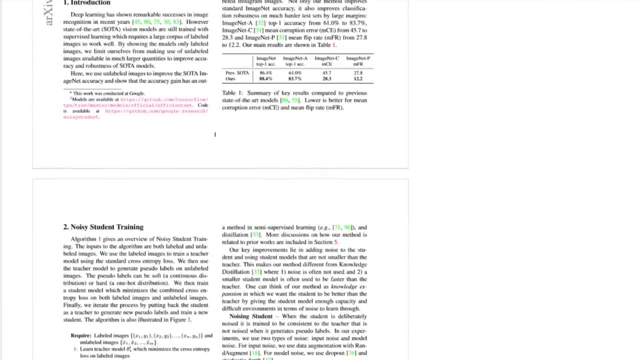 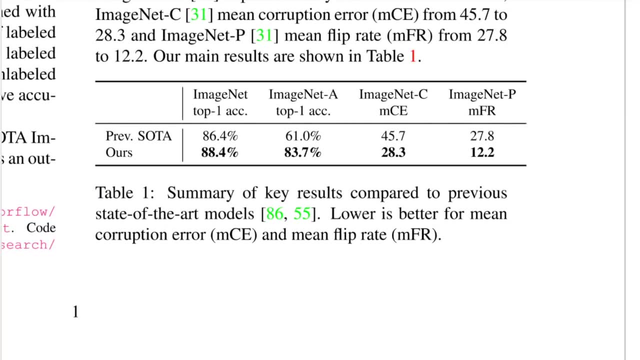 know, Okay, this, this is basically it And, as you can see, this is kind of their main final results, where they say: on ImageNet, our top one, accuracy sort of increases right here, And even on these kind of subsets of ImageNet or these are sort of corrupted sets of ImageNet, they 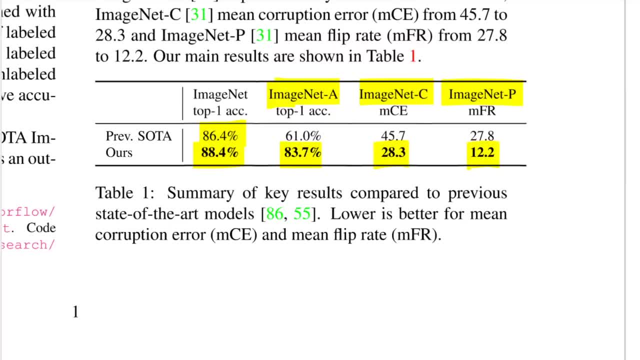 make even more substantial improvements, as you can see here. Now we'll go into what these corrupted subsets are, But no, just for now. these here are very difficult variants of ImageNet. Other models are most commonly used in comparativelyobilized modeling center, So this over here is an example. 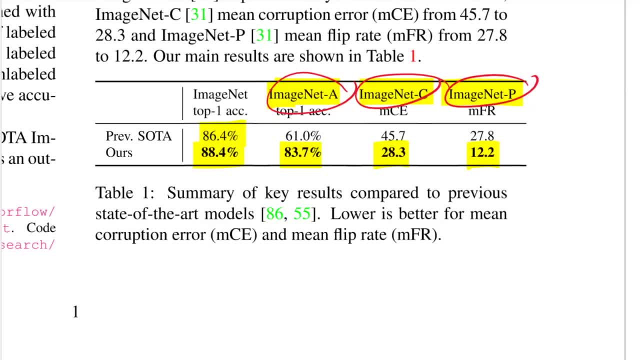 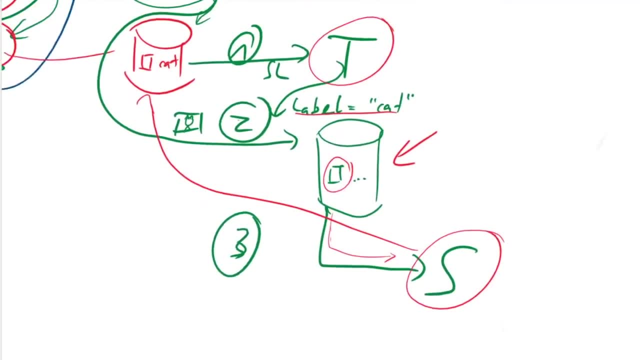 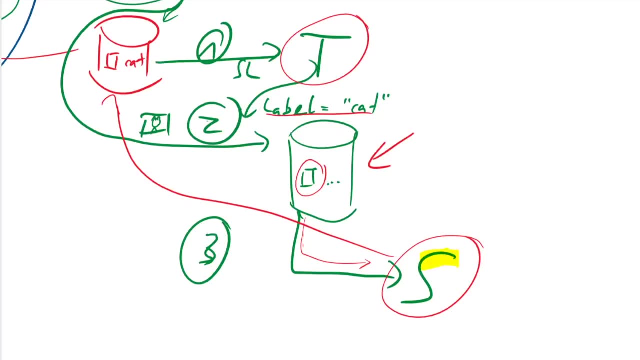 of an example where this one can be severely corrupted or or distorted and so on, And you can see that the model improves severely over the previous state of the art, which basically means that this model is more robust, and that's a direct consequence of the noise. 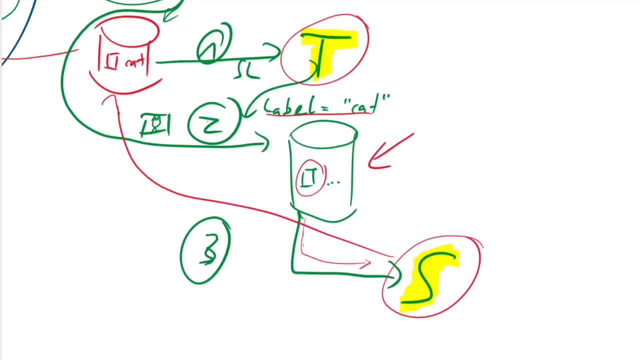 Now, one last thing I should say Is that, as a model, as the architecture, So in combination with the noise, right here, with the noise in combination, that means the student model is probably able to capture more of the variance of the data. it's larger, it has more parameters, it can learn more about the data together with the. 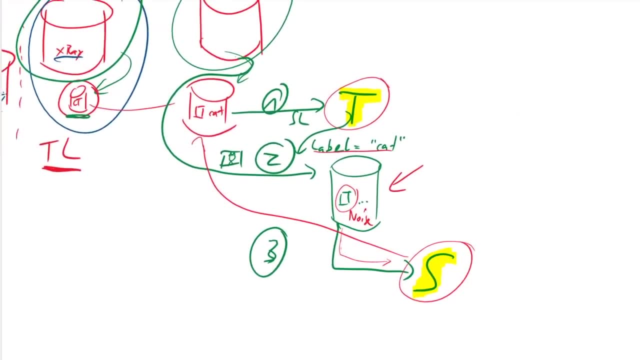 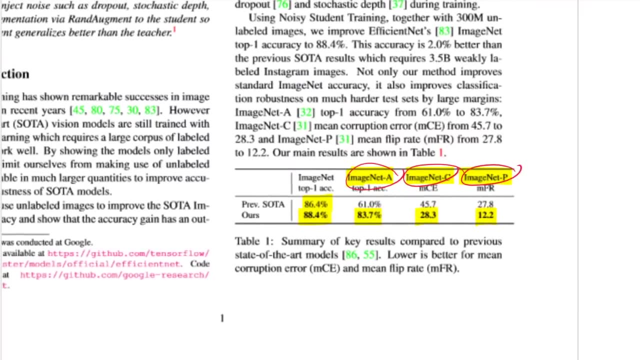 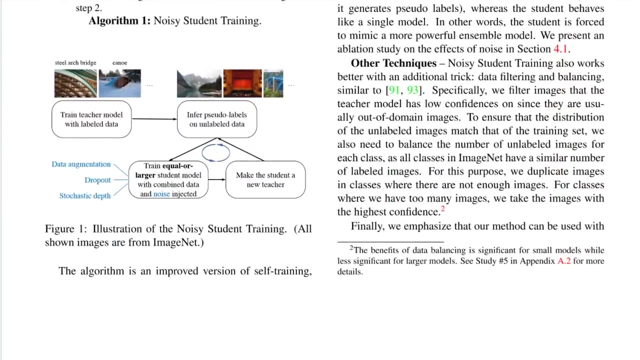 noise, it can probably be more robust And that's what makes it generalize better And we'll also see, as we see here, it's more robust to these transformations And it's also going to be more robust to adversarial perturbations. So the the technique again is illustrated here as, as we 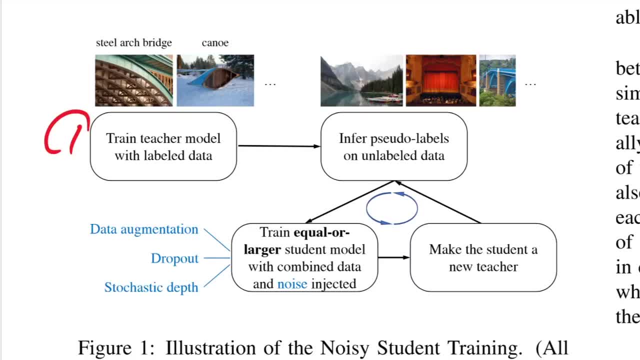 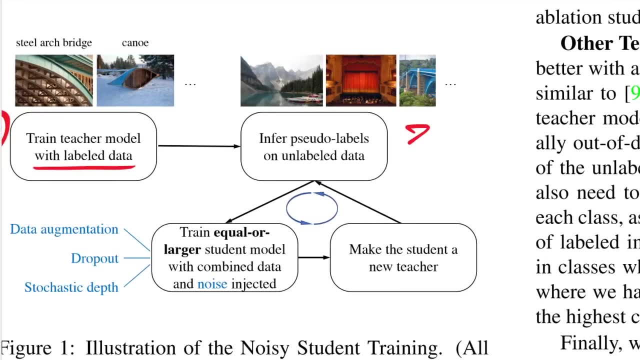 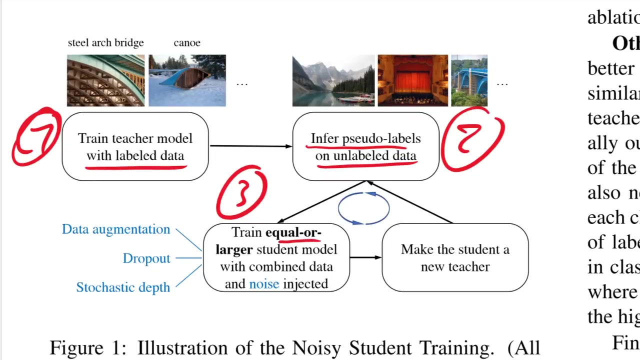 said it's pretty simple First. so step one. step one: train the teacher model with labeled data, as you would. Step two: you infer the pseudo labels on unlabeled data. Step three: you make a student. you make. sorry. we'll step three, over here: train an equal or larger student. 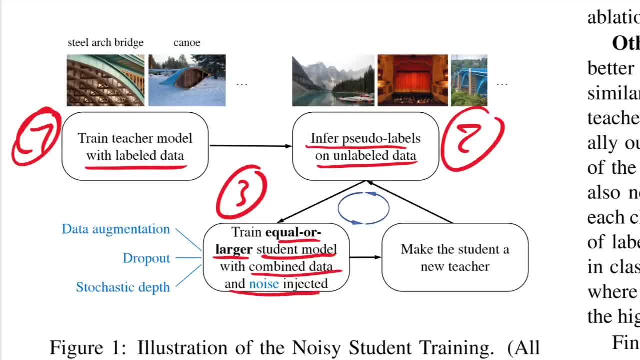 model with combined data and noise injected. So they don't. they use the original labeled data here and the pseudo labeled data right here in order to train the student, But still this: the student doesn't have more information, more label information than the teacher had, it simply has. 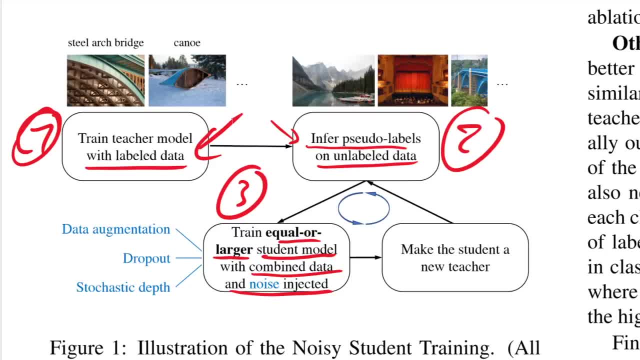 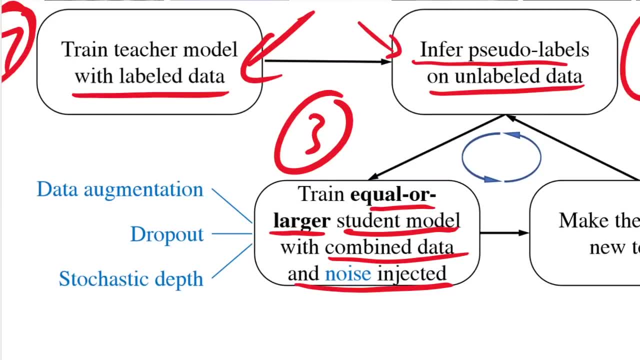 this teacher labeled unlabeled data, also to train on. Now, the crucial part here is, well, first of all, that the student can be larger And, second of all, that there can be noise, And the noise comes in three different forms. So, first of all, you use data augmentation, which we've already seen. this is 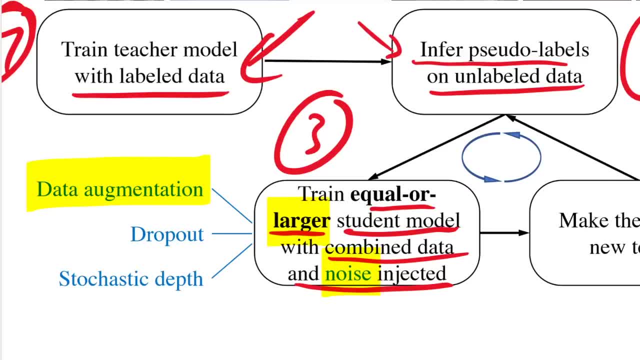 sort of like random cropping or mild rotations, color jitter, whatever. they use a rand augment here, which is a specific technique to apply these augmentations. They use dropout, which is a fairly old technique, where you, in the student model that you train. 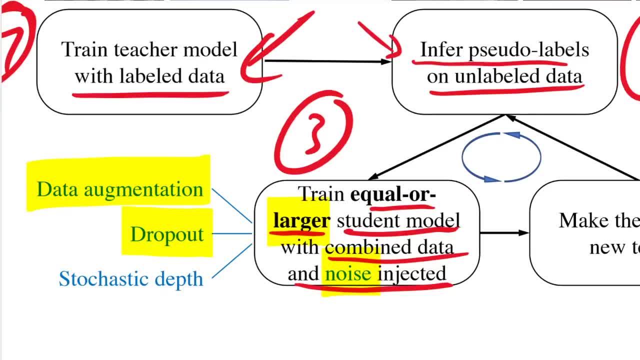 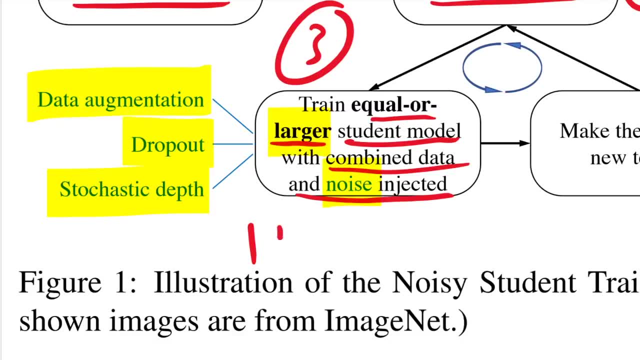 you randomly drop out connections, which makes it more robust and more generalizing. And then you also use stochastic depth. Now, stochastic depth is a technique when you train a model, what you'll do during training, instead of always passing your data forward through the layers, like 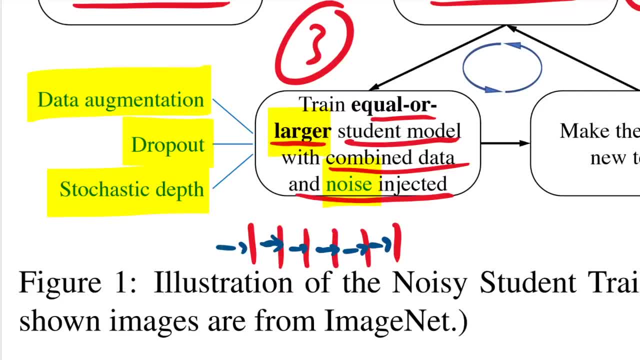 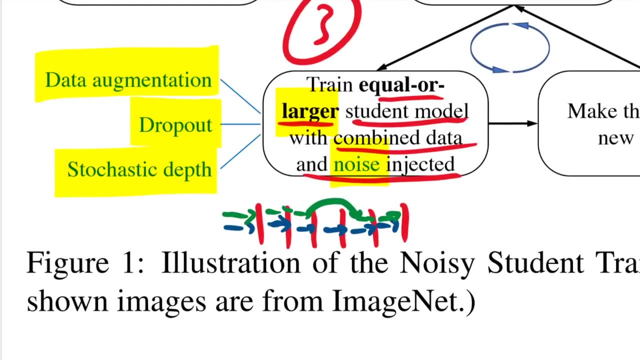 this. you use some sort of a dropout, but with entire layers. So what you'll do is you'll pass your data forward and then, randomly, you'll skip a layer and then pass it forward again. Now, these these might seem weird first because, yeah, it might seem weird, But 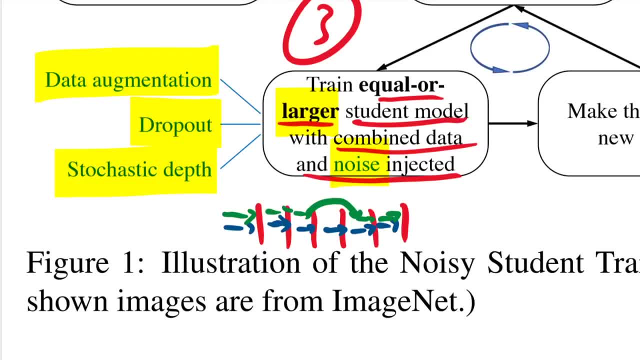 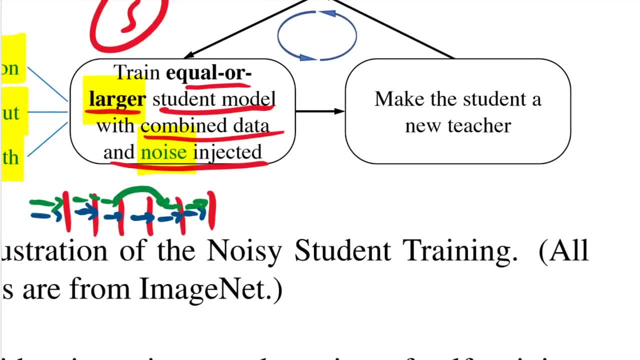 in if you know that most models, especially computer vision models nowadays, are residual networks, which means that their layers look like: so you have the input, you have some computation and then you have the output, And then there is already a residual connection that basically adds the original signal together to the result of the 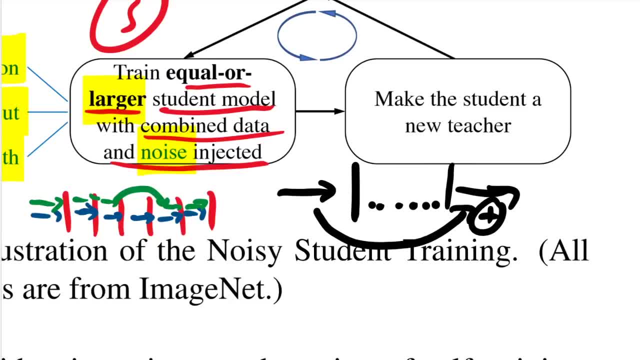 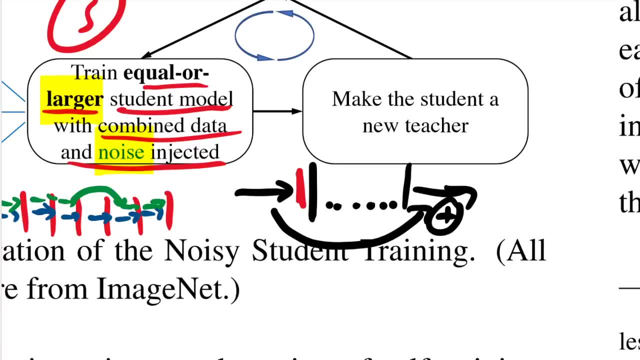 computation. So all you do in this stochastic layer dropout or this stochastic depth right here, is you basically disable use, you disable this connection right here and all the signal has to flow through here. If you read the residual, the ResNet original ResNet paper: 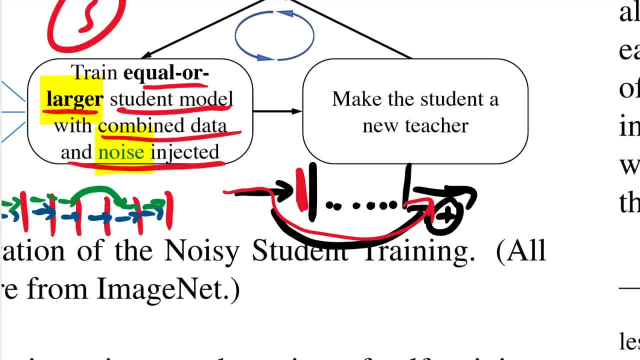 they make it pretty clear why the residual connection is a good idea. Basically they say: these computations, here they: if you have a very deep network, each layer only has to basically do very little bit of computation. that that can be bypassed fairly. 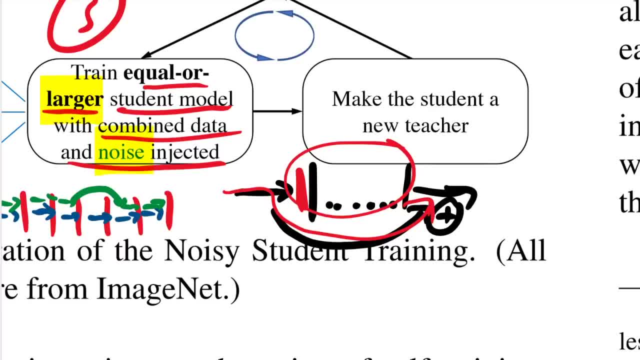 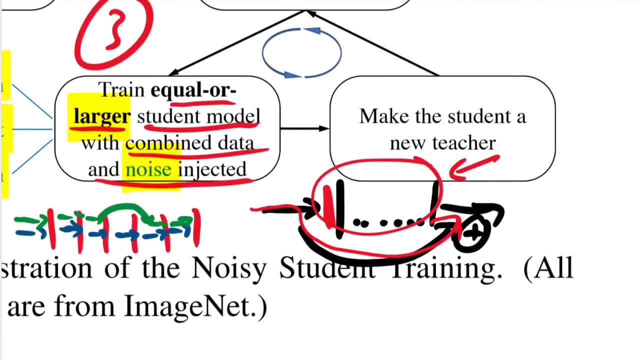 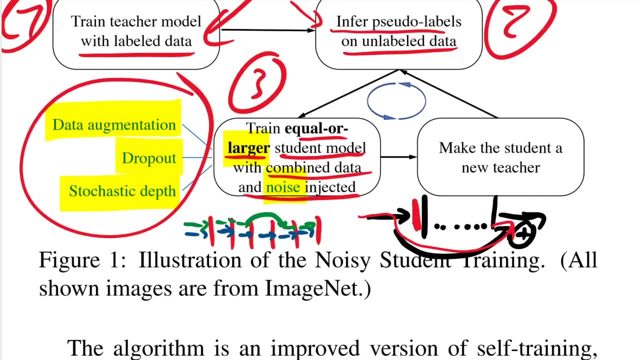 efficiently for a lot of data points. So it's not that hurtful to bypass a layer, And in this case they actually use it to just bypass some of these small computations and inject some more robustness into the student model. So with these three strategies to bring noise into the training process- one is on the data- 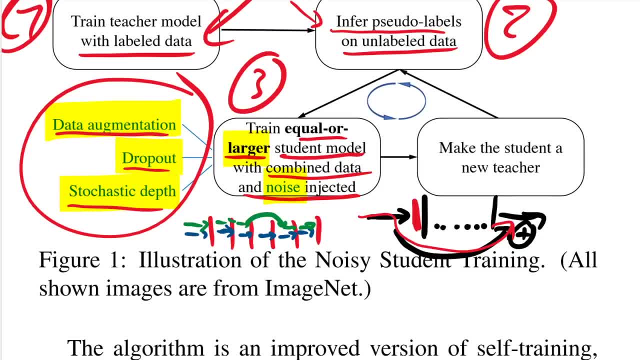 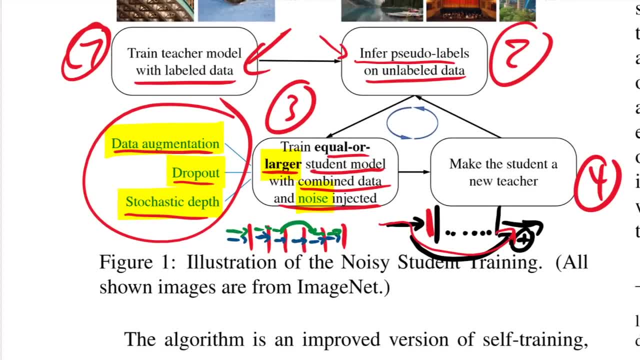 and two is on the student model itself. they train the student model. and then fourth- and this is what we didn't have before- four, or maybe we put four here. make the student a new teacher. So now you can iterate, you can use the student model that you just trained. 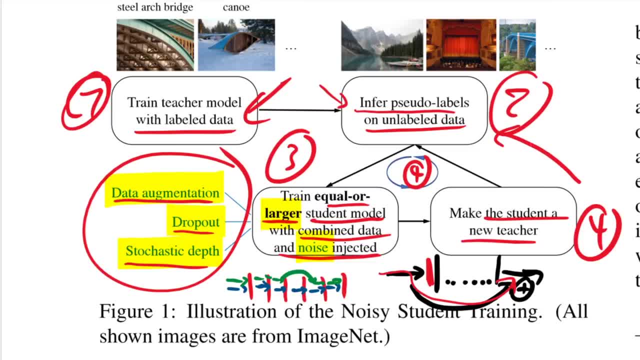 to again label the unlabeled data, And then you can use another student model, again under the influence of noise, to train from that student model, and so on, and you can go on, And they do up to like three iterations of this where 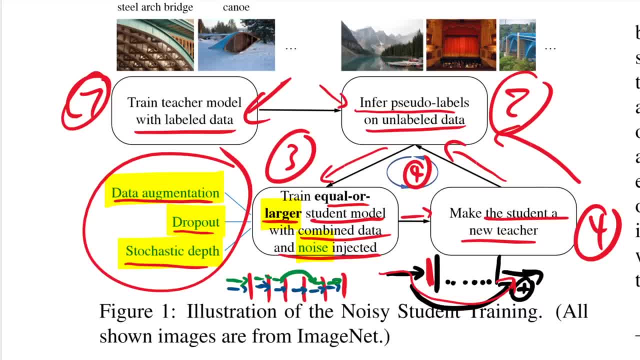 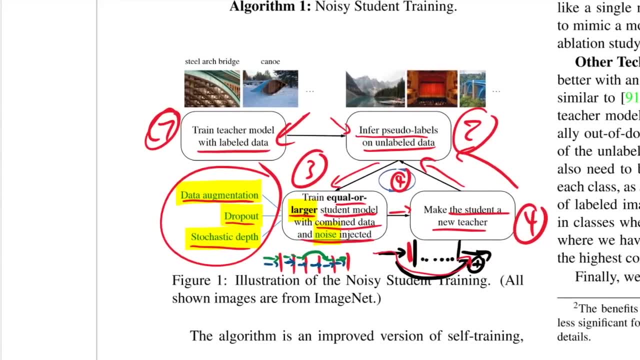 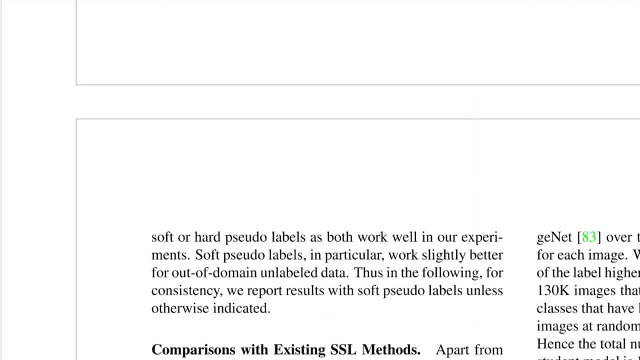 they always take the new, the student, as the new teacher and then use a new student model to train from that teacher, And they get better and better as they do this. of course, there's like a diminishing returns, but it's pretty impressive that this even works right. So 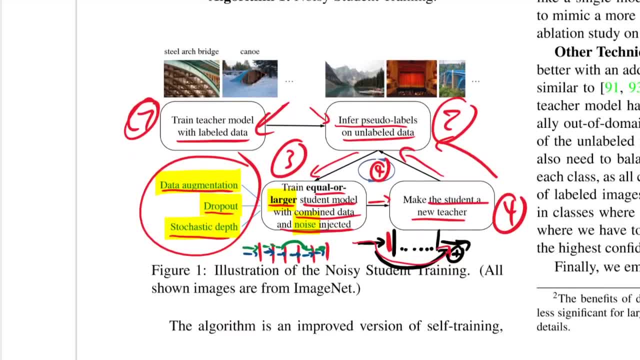 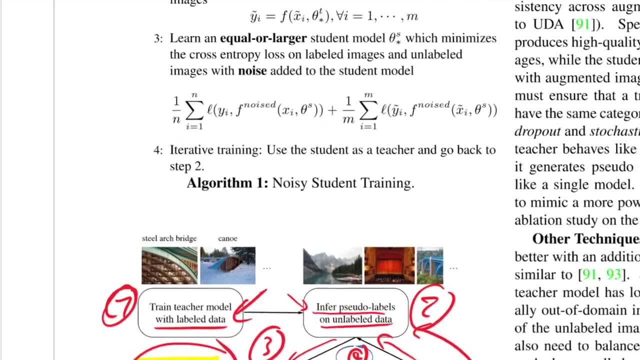 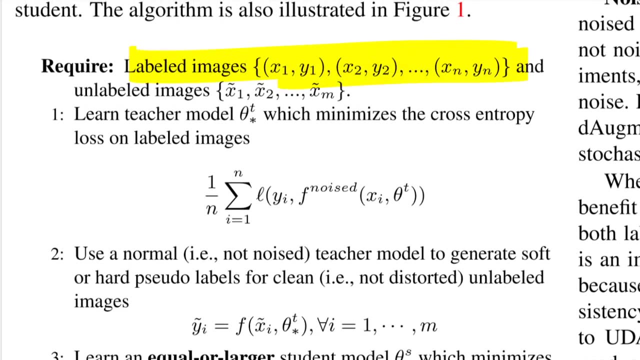 the new students in fact aren't even larger than the old students. it's just that the students are larger than the original teacher model in most of these cases. So here's the algorithm written down. you'll require labeled images right here and unlabeled images, which. 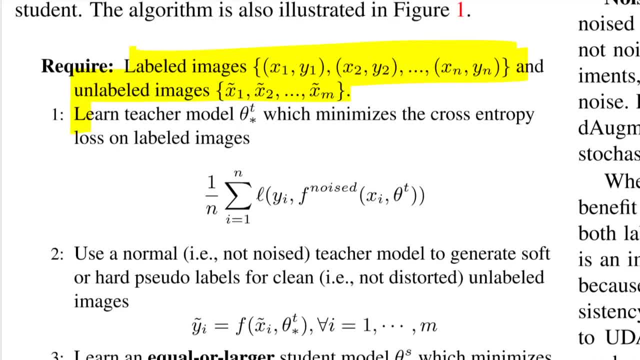 are the ones with the tilde. So first you learn the teacher model, which minimizes the cross entropy on labeled images. this we already know, this right. This is the label, this is the image according to the label, And you train the teacher model. 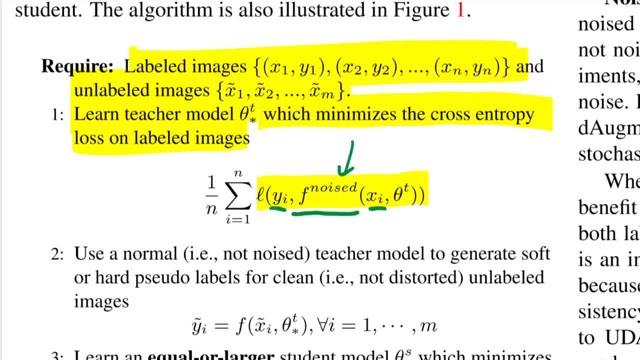 which is this thing here And you can see here noised. So already in the teacher training process. you want to introduce this noise, you want to introduce these data augmentations. These are, as I said, these are standard techniques to make models more robust and therefore more generalizable. 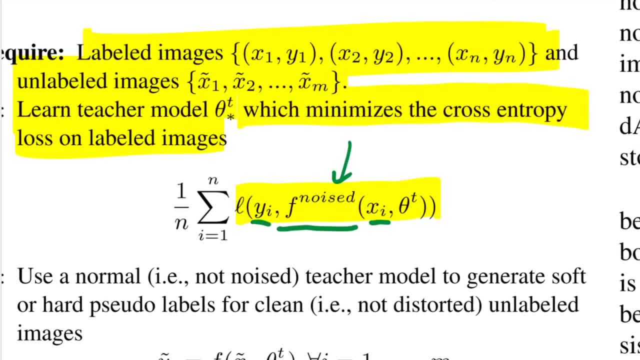 Yeah, we know from these, from the self supervised papers, that these augmentations are very powerful and the way you design them. basically, if you one of these augmentations is a random crop, which means if you have an image, you randomly crop out like part of that image and then that's. 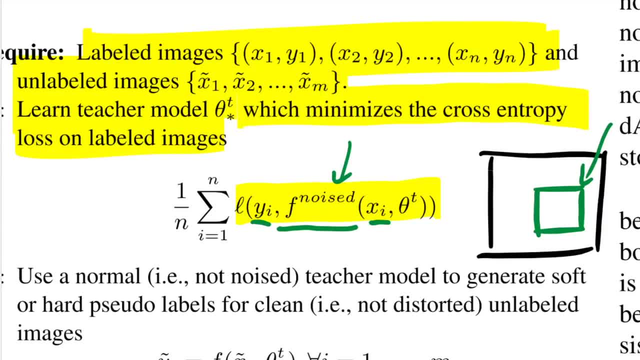 your training sample and not the entire thing. So by doing this, you basically teaching the model to ignore the exact location and scale of things on an image, And you can do this because you, as a human, know that. you know I can zoom in, I can zoom out into something and it won't change. 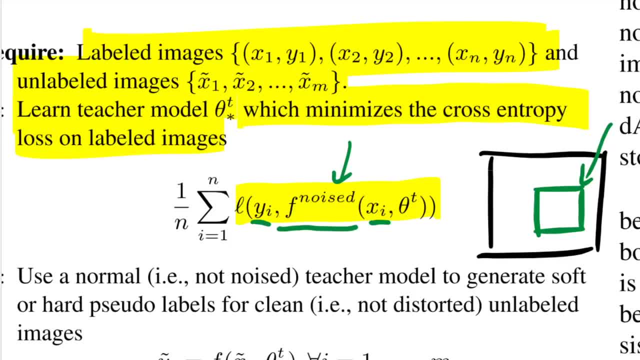 what's on the picture. And so that's, you use these augmentations to kind of heuristically tell the model what it should be invariant to, And that is. that is a very powerful technique to regularize, basically to to robustify these deep, deep methods, And this is used the same here. So 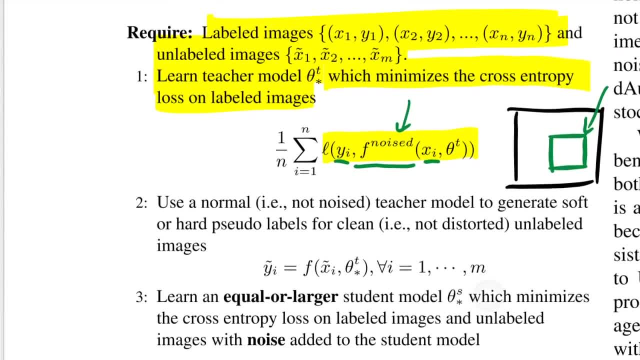 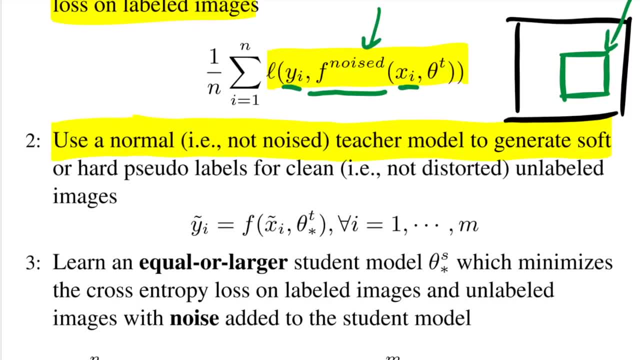 already in the teacher model we train with this noise. And then, step two, use a normal ie, not noise, teacher model to generate soft or hard sudo labels for the clean ie not distorted on enabled images. And this is important, they stress this here- that when you, when you label the unlabelled, 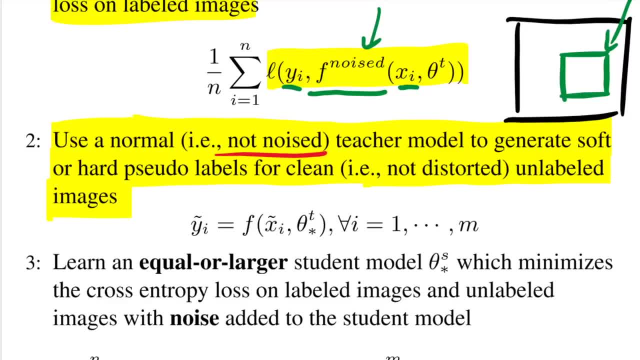 images. you want to use the model that is, without the noise, and you do it on the not distorted, unlabeled images. So when you infer the labels, it's very important that you have clean, accurate labels without any sort of a noise in them. So labeled images are used when you write the pvc or labels are used, in other words on speechués, And so you kind of get a way of leaving your work clean, accurate labels without any sort of noise in them. So labeled images are usually done by you when you're creating fairly complex dc macros. So what I've learned in my class, of course. 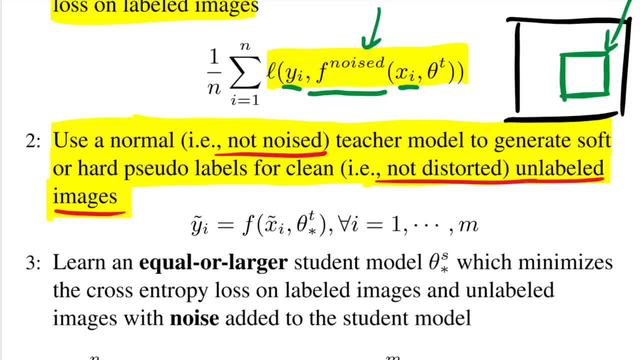 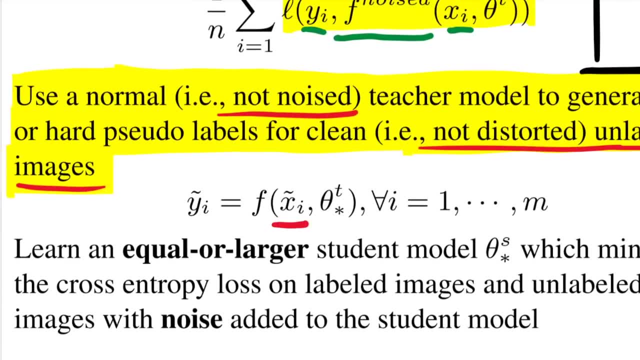 and your model. probably the fastest step is to define certain things that you should avoid, and label noise is not something that they have found to help in this case. So not label noise on the teacher. that is So you can see right here on the unlabeled images. we'll use that teacher model. 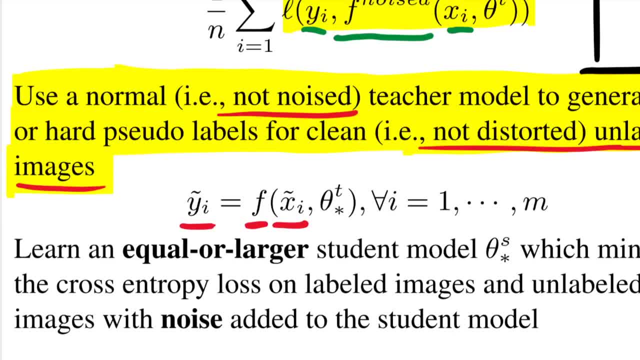 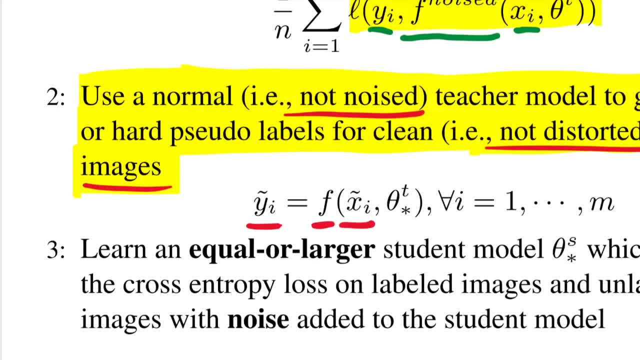 without the noise to infer the labels. Now they say these can be hard, model hard labels or soft labels. So what does that mean? If we generate hard, pseudo labels, that means that the Y here is simply going to be either zero or one or two or three and so on. So just the index of the class. 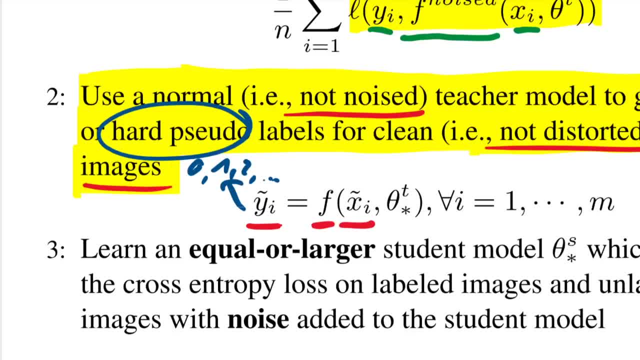 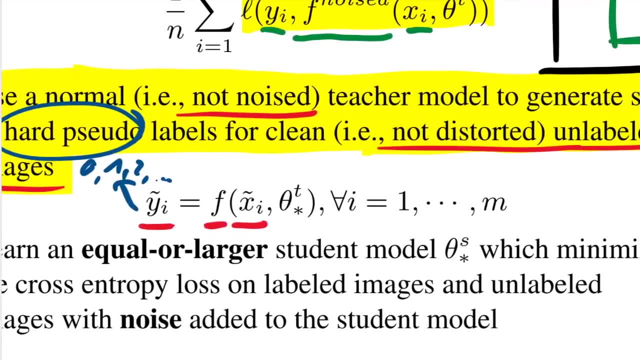 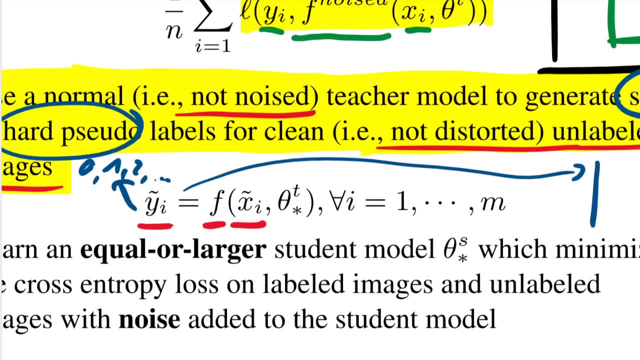 whichever class is most likely. that's going to be our label. This is exactly how the supervised data sets come right. So this is what you'll think first when you see that, However, soft pseudo labels means that the Y will be a distribution, So instead of being of class zero, it will be sort of 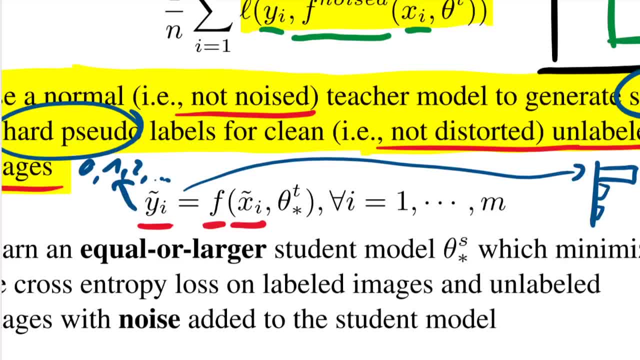 let's say, 90% of of class zero, but also 5% class one and 5% class two. right, So you'll output the distribution instead of the just the label. And they have found that the soft pseudo labels work slightly. 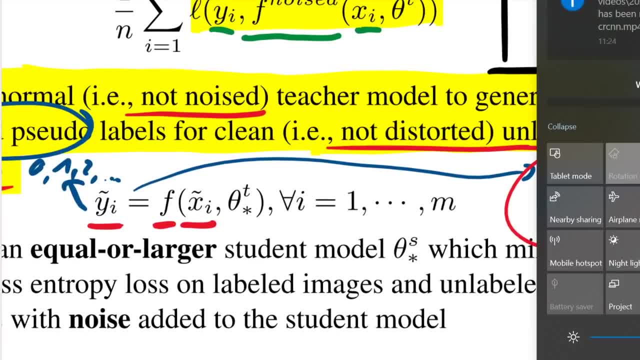 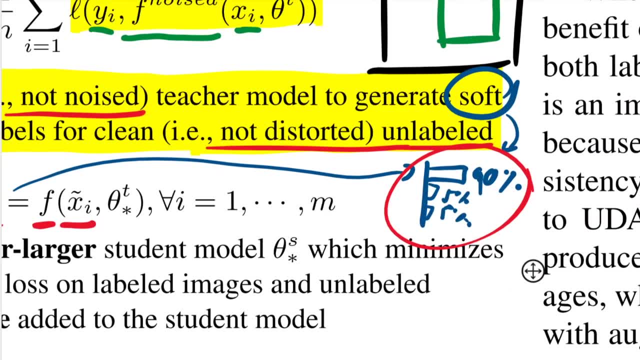 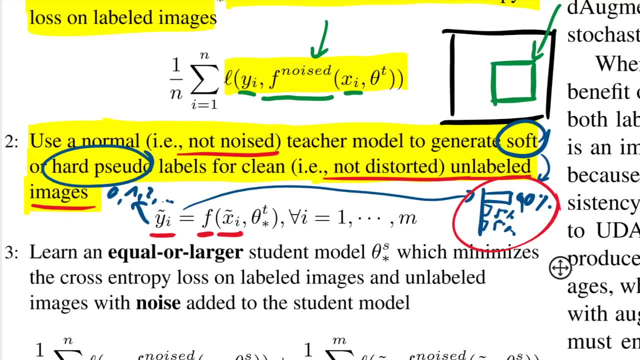 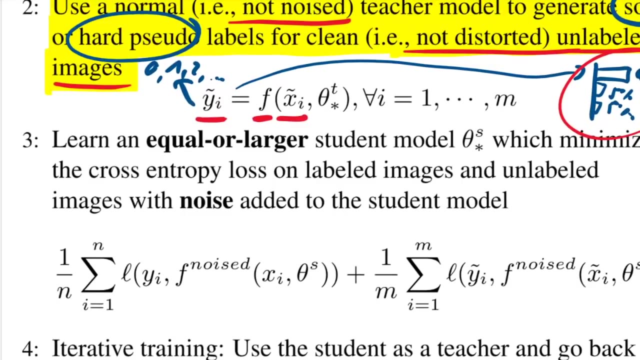 slightly better than the hard pseudo labels. Okay, thanks, So that they use the soft pseudo labels here because they work slightly better. but you can do it with hard or soft labels. The important thing is that you use the teacher to generate as accurate as possible labels for your unlabeled data. Then, third, we've already seen this: 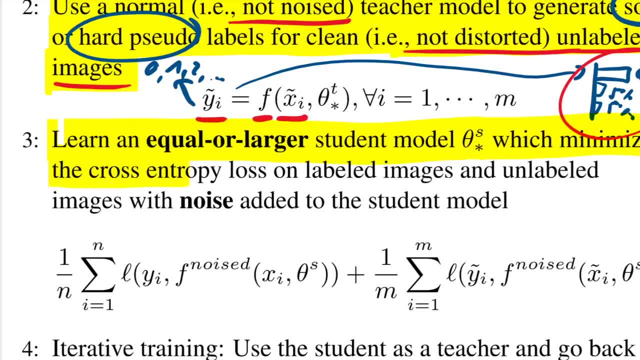 learn an equal or larger student model which minimizes the cross entropy loss on labeled images and unlabeled images, with noise added to the student model. So, as you can see, labeled images and unlabeled images. So we're in this semi semi. 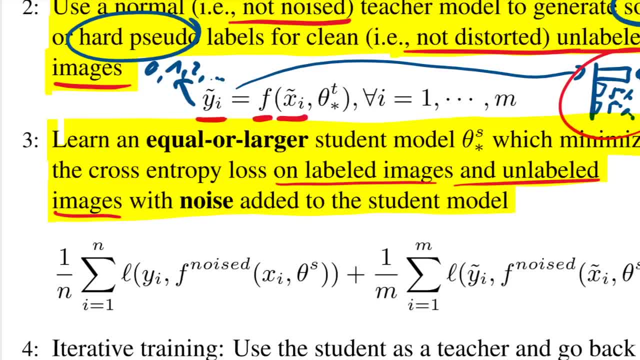 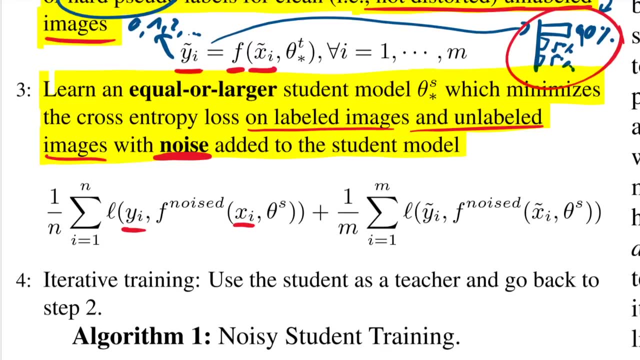 supervised learning setting. right now you take in both together with noise, and noise here is in bold, which means they stress it again. this is important, So you can see that the loss is composed of two different things. These are the true images of your original model, And you use that And this. 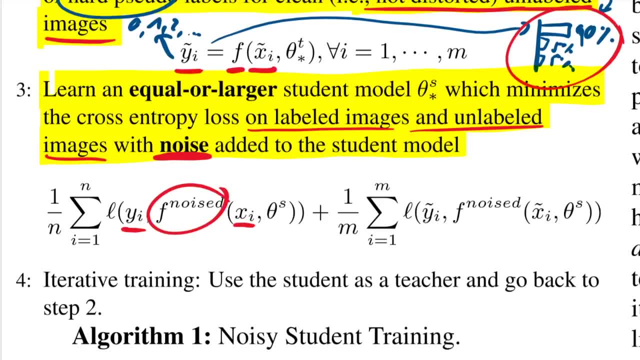 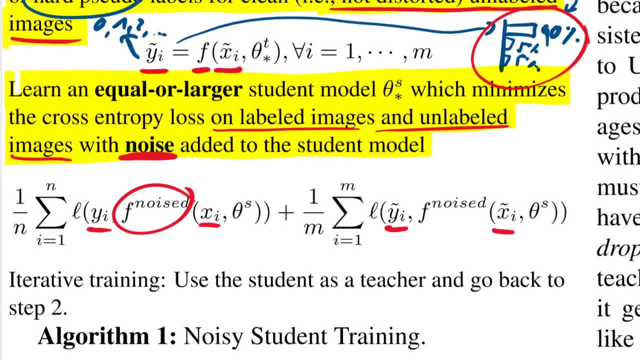 means you noise the student model, And that noise can be on the data or in the model itself, And here also the unlabeled images that you have labeled with the teacher. you do the exact same thing, So you train on both of these data sets. 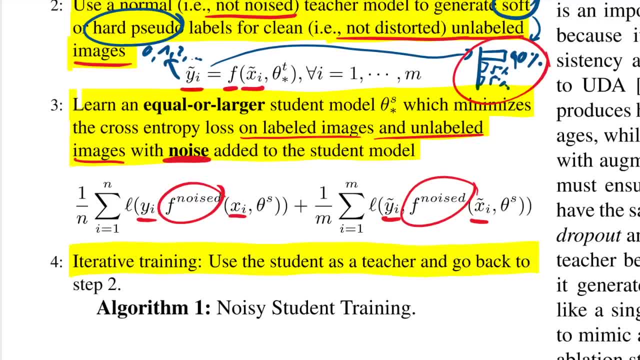 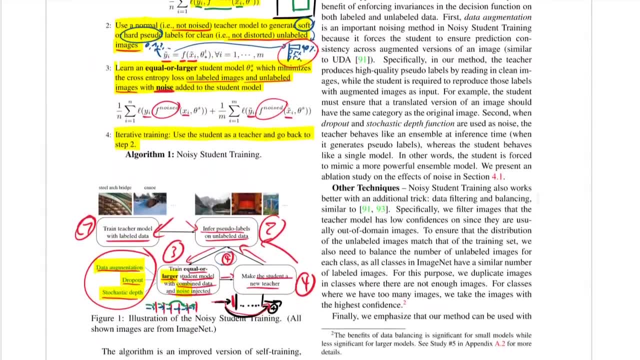 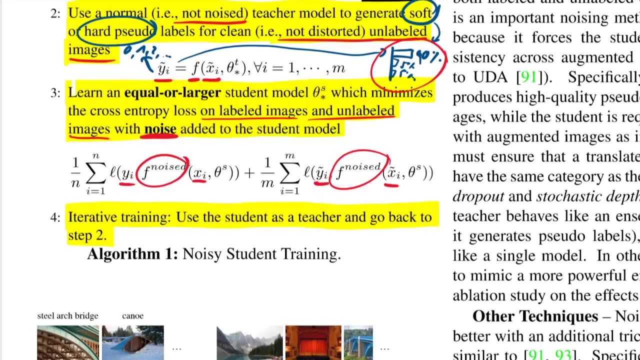 And step four is: if you want to do iterative training, use the student as a teacher and go back to step two. Now they have some more tricks when they do this iterative training. They also up the batch size during the iterative training and so on. So they do a lot of things to make the student. 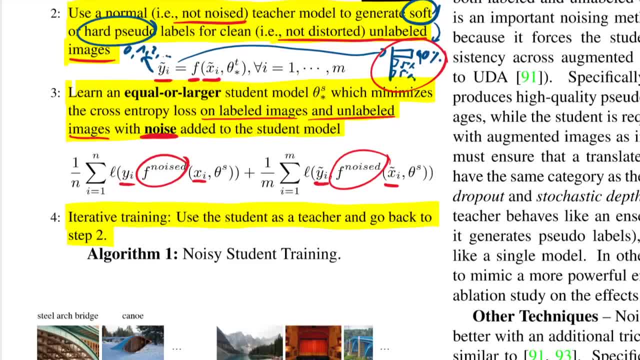 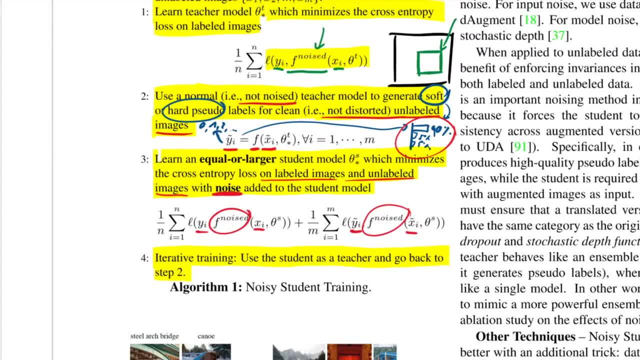 learn something more, something better than the teacher. And I think this the whole paper. it doesn't- it doesn't state it explicitly, But I think the whole paper. everything they do here is to kind of force or allow the student to become better than the teacher by by giving more noise. 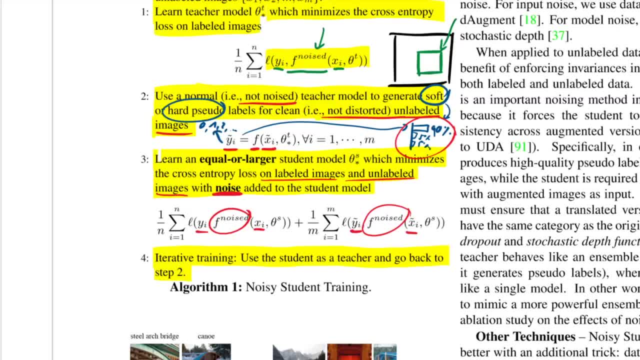 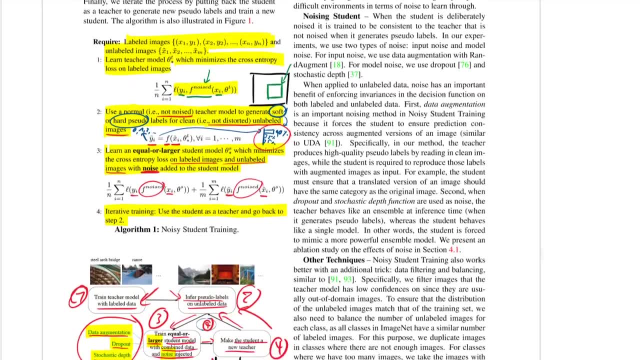 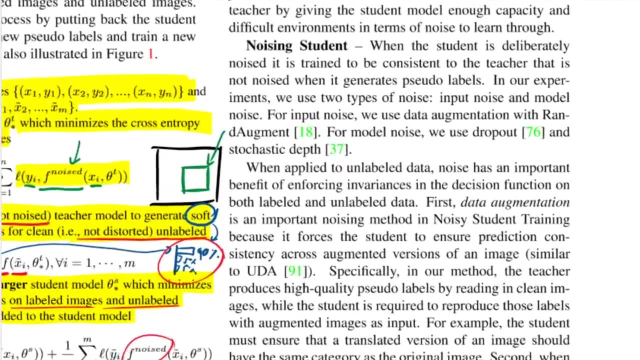 by making the student larger, by making the batch size for the student larger and so on. So you want to sort of inject as much in variance as you can and that will make the student learn more. So they say here: noising student, when the student is deliberately noised in its 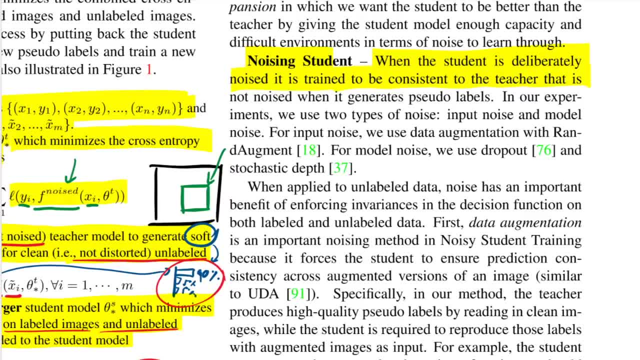 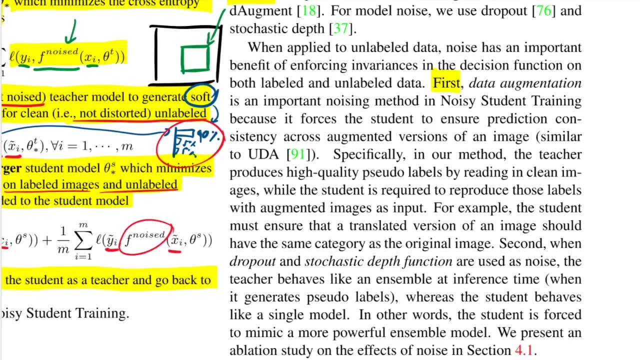 it is trained to be consistent to the teacher, that is not noised when it generates the pseudo labels. In our experiments we use two types of noise: input noise and model noise. All right, First, data augmentation is an important noising method. in noising, 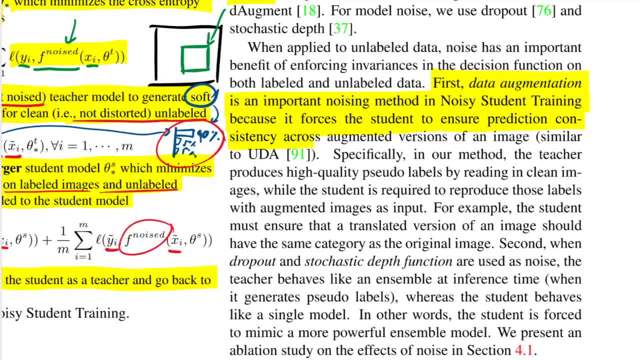 student training because it forces the student to ensure prediction consistency across augmented versions of an image. Specifically, in our method, the teacher produces high quality pseudo labels by reading in clean images, while the student is required to produce, to reproduce those labels with augmented images as 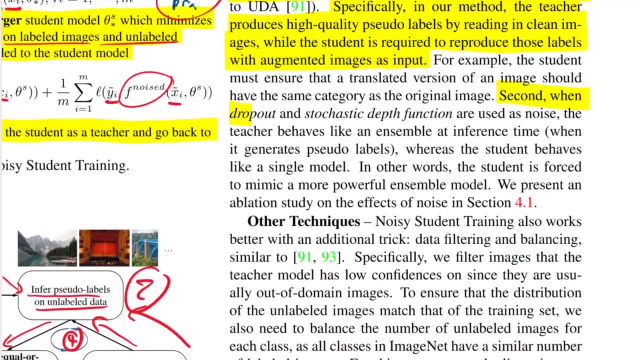 an input. Second, when dropout and stochastic depth function are as noise, the teacher behaves like an ensemble at inference time, when it generates pseudo labels, whereas the student behaves like a single model. In other words, the student is forced to mimic a more powerful ensemble model. we present an ablation study, So this, it's a bit weird. what? 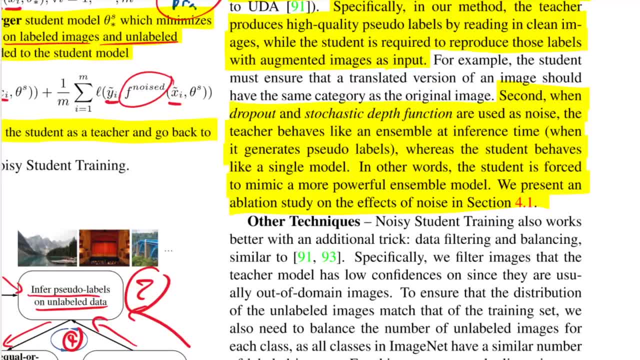 they say: here, Don't be confused, you use the dropout and the stochastic depth on the student model. And they say: here, if you do this, the teacher behaves like an ensemble at inference time, whereas the student behaves like a single model. And yeah, it's. it's a bit of a weird formulation. 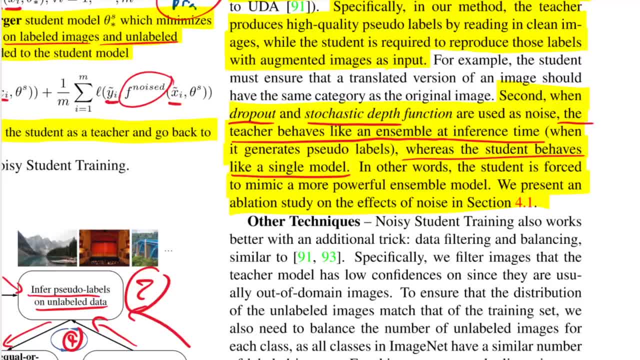 But it's it's true like the teacher, the teacher will produce these same the label for different pathways through the students, if you use dropout and kind of stochastic depth, And therefore the student is kind of required to approximate each time each forward pass has a different forward pass through the layers, through. 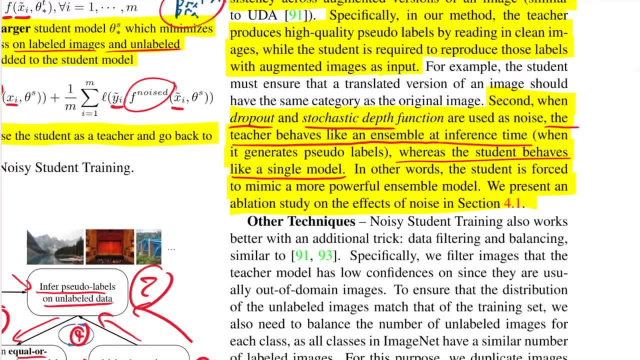 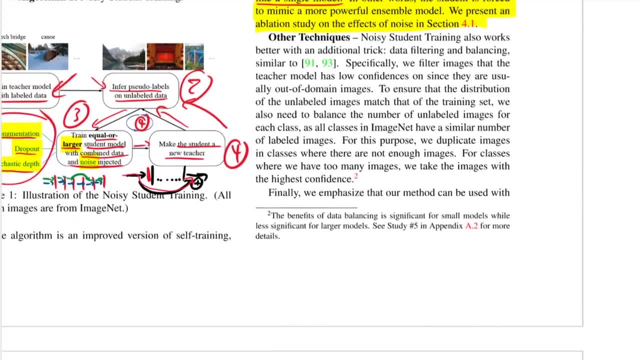 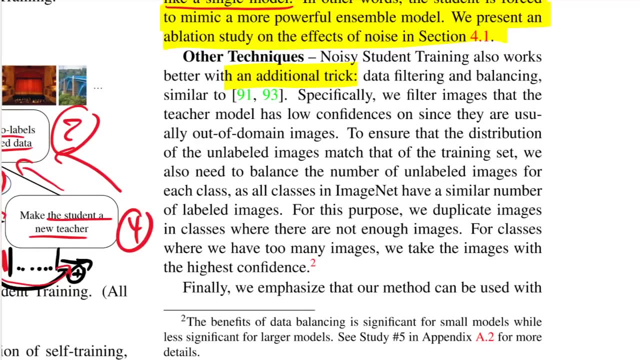 the connections with dropout, And it's forced to approximate that teacher label with all of these different things. So you see that you, you put in a, lot, of, a lot of techniques. so they have even other techniques. There is one additional trick, and it's not an, it's not one, actually they have. 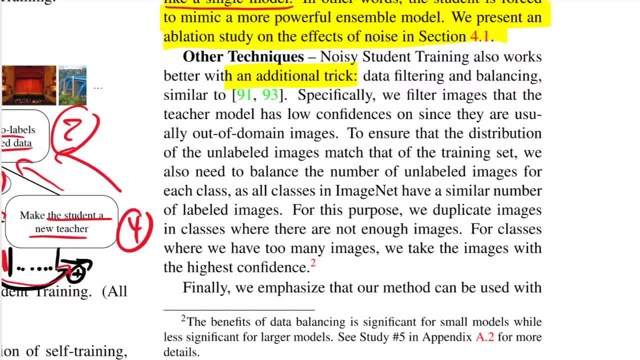 so many tricks And if you look at their experimental setup that it's crazy. Like they describe exactly, we reduce the learning rate like this, and the batch size like this, and so on. So to get state of the art on ImageNet, it's not enough to just have a good idea of a new thing. to do what? 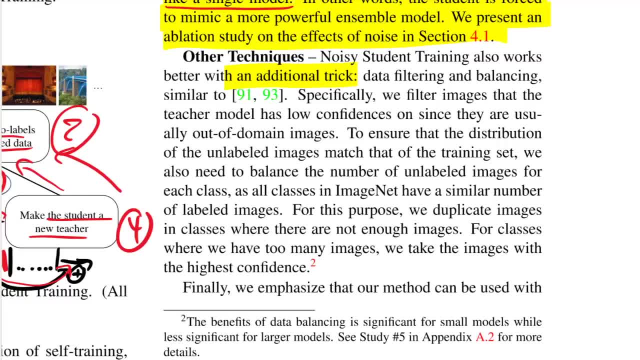 you. you have to have the good idea and then execute it almost like really well, Because you have to regard all of these additional tricks that people have figured out over the years. In any case, they say it works better with an additional trick And that is data filtering and balancing. Specifically, we filter images that the teacher model has low. 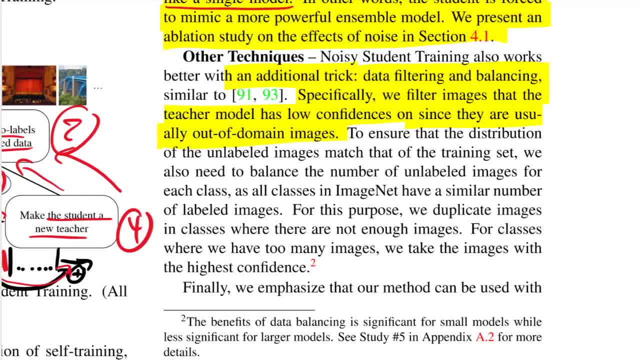 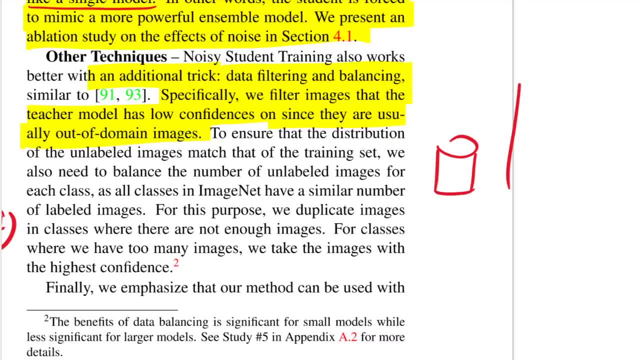 confidence on, since they are usually out of domain images. So that goes to a point where, if you see, we have this ImageNet labeled data set, right, and we have the larger data set. Now, the larger data set simply contains images and there is no guarantee that the images are actually of the classes that we have in the 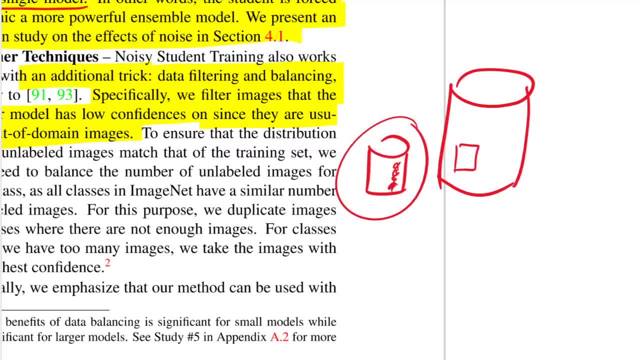 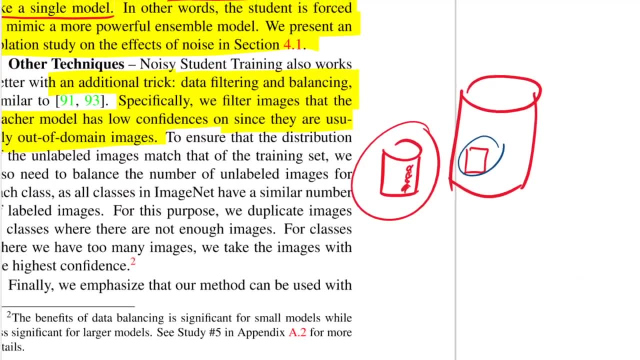 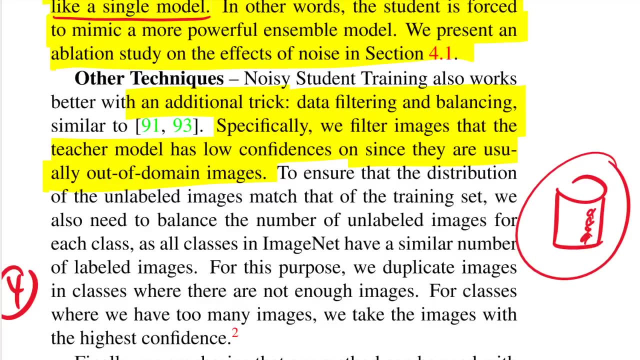 ImageNet data set right here. we have 1000 classes here. There's no guarantee that these images fit into any of those classes, Yet we still ask the teacher model to put them in some of these classes. Now you can filter out part of those images If you can look at the teacher model and you look at its 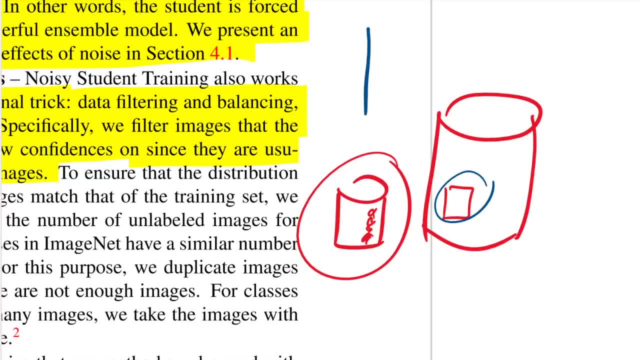 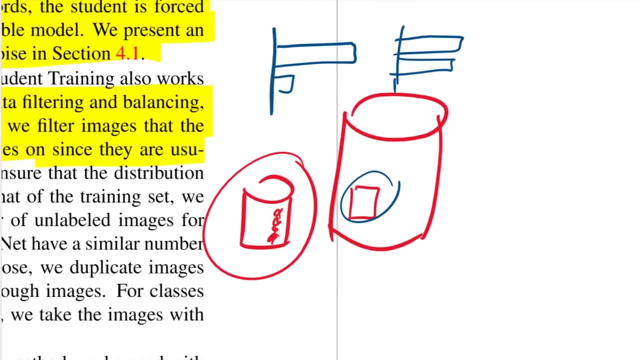 confidence. so when it outputs a distribution, if, if there's just two labels, let's say, if it outputs a distribution like this, that's wildly different than if it outputs a distribution like this. Both are class one labels, but one is much more confident than the other. So what you want to do is you want to filter out these low. 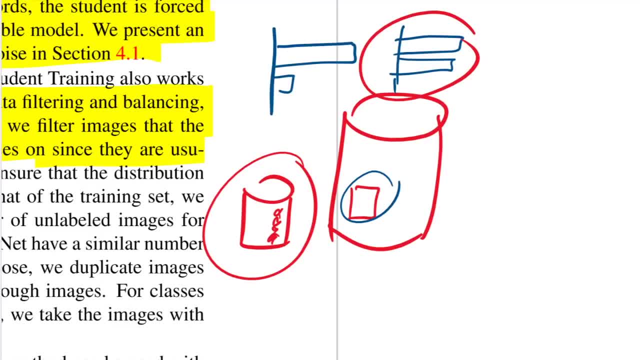 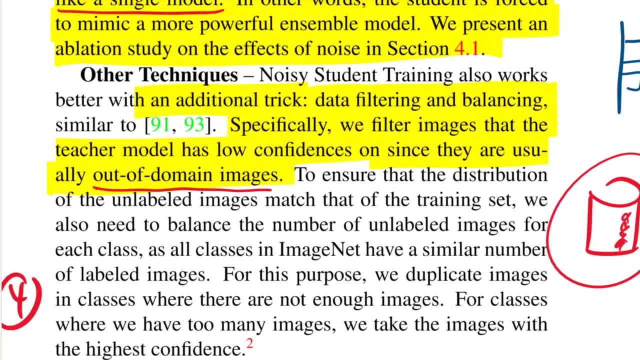 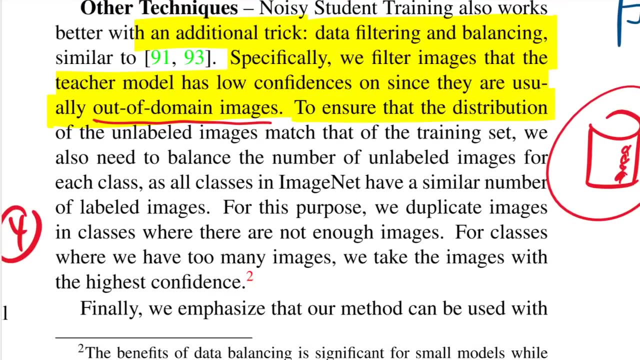 confidence labels because you know the model isn't really sure but it has to assign a class, But that's usually an indication that it is an out of domain image. So if they filter this it works better. And then also to ensure that the distribution of the unlabeled images match. 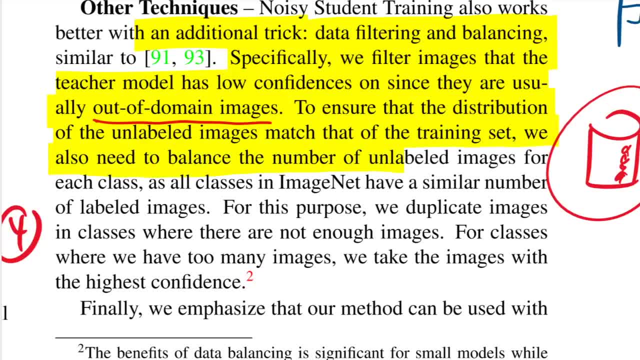 that of the training set. We also need to balance the number of unlabeled images for each class, as all classes in ImageNet have a similar number of labeled images. For this purpose, we duplicate images in classes where there are not enough images. For classes where we have too many images, we take the images with the 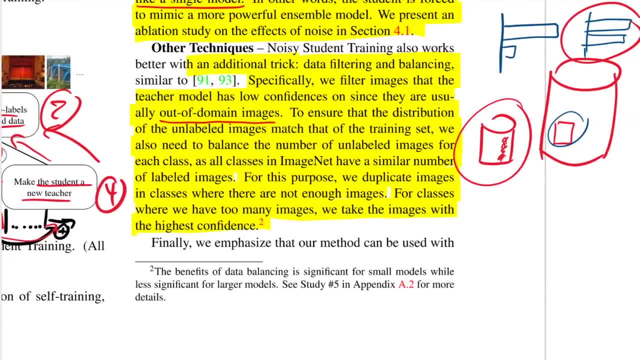 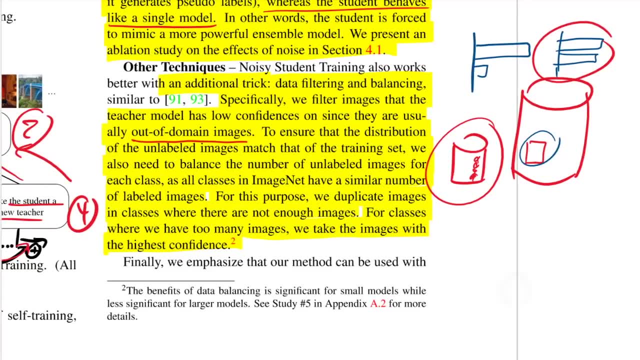 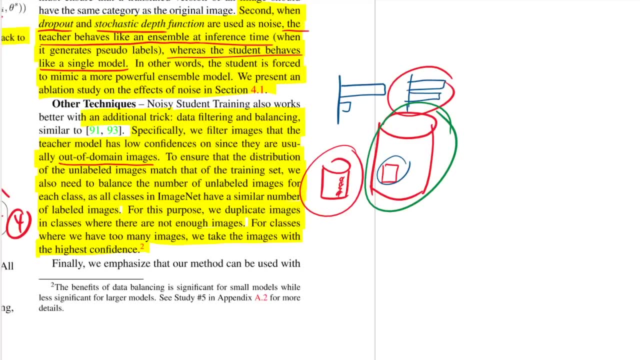 highest confidence. Okay, so this is just another technique. this has basically nothing to do with their core idea, But this is just another thing where they say, Okay, we can treat this big thing that we scraped from the internet, you know, we can somehow filter and balance it smartly and that will work even better. 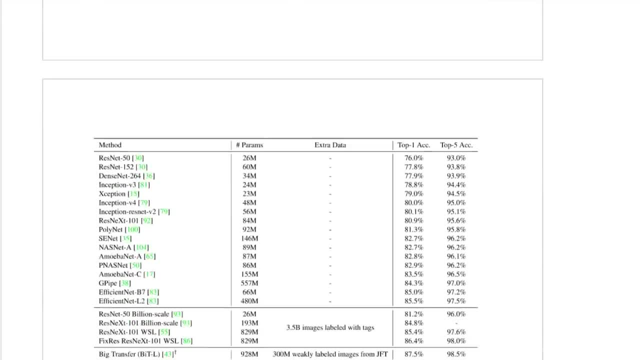 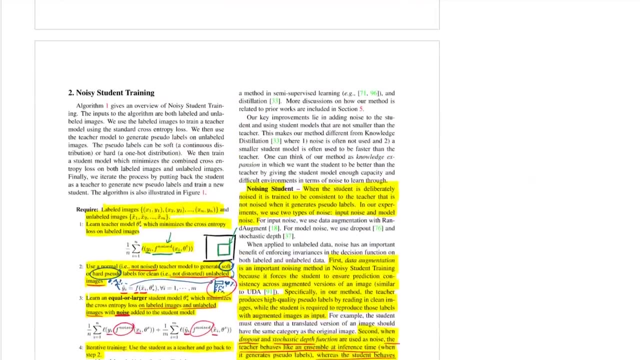 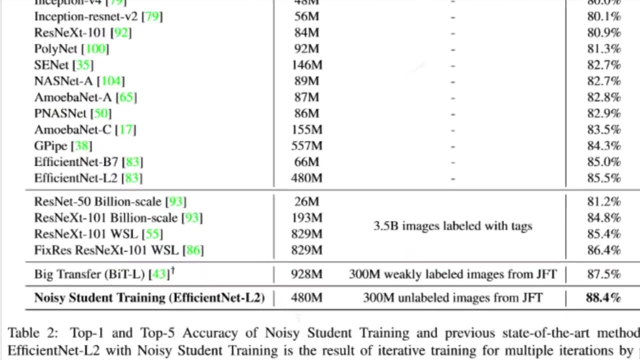 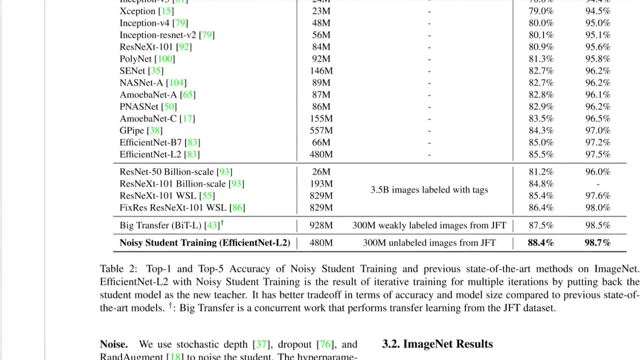 Alright, so let's go into the experiments, Of course there. So what they do? I think where is the graphic? what they do is they take an image net- sorry, they take an efficient net right here And they trained. they first train an efficient net, a smaller efficient net, as we said for to be the teacher, and then they train a larger. 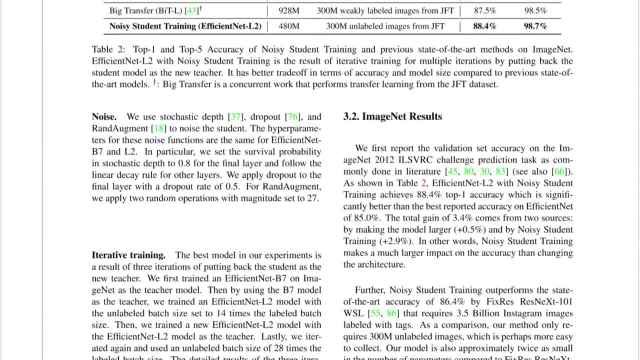 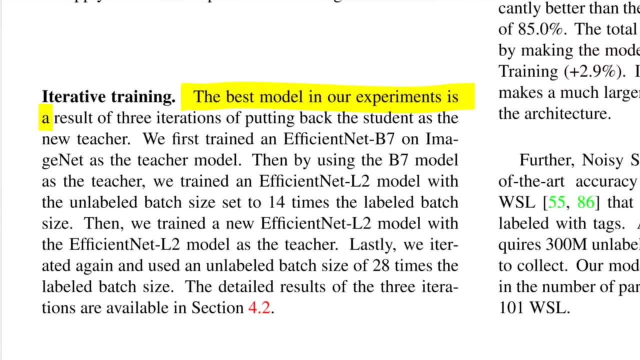 efficient net for the student. The best model in our experiments is a result of three iterations of putting back the student. as a new teacher. we first trained an efficient net B 7 on ImageNet as the teacher model. So you can see in the table right here what the B seven achieves. The efficient net. 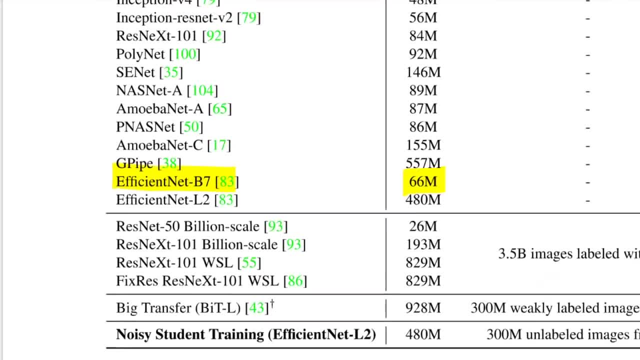 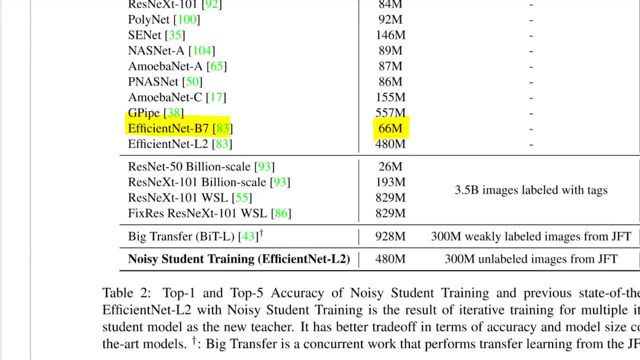 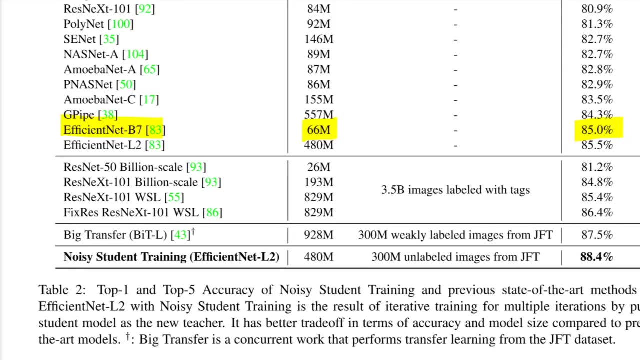 B seven. here you can see it has 66 million parameters, which is fairly small compared to these other kind of previous state of the art methods on ImageNet, right? So they first train this and that will achieve something like an 85% accuracy. Now, if you just train a larger model, 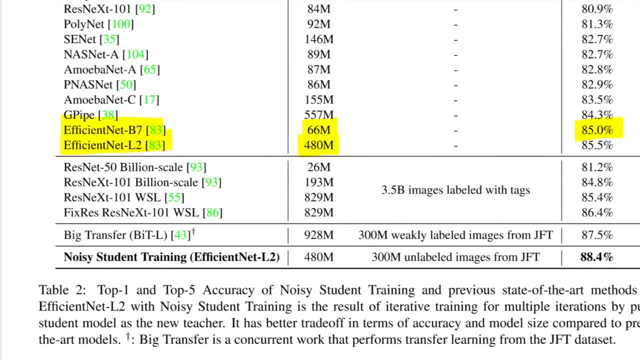 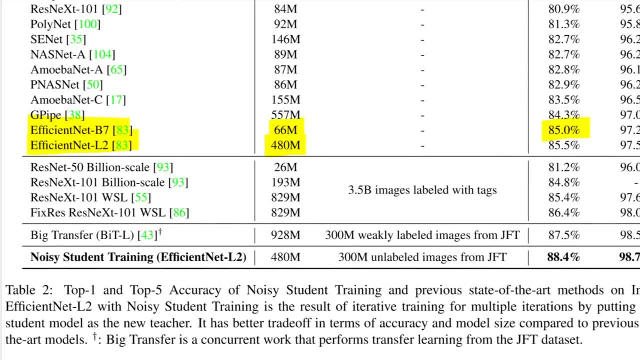 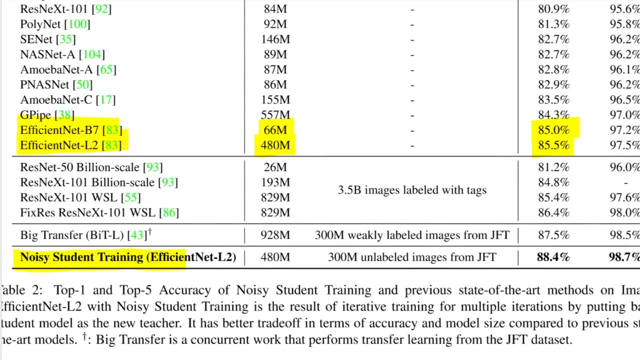 this efficient net L two right here that has, you can see 480 million parameters, so a lot of more million parameters. but you just train it on the same data set on ImageNet you will get a 0.5% improvement. And you can see that here with noisy student training with the exact same model. 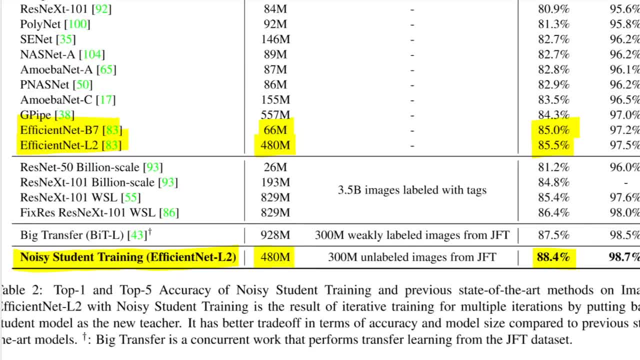 so it has the same amount of parameters, you'll actually get an 88.4.. So I like a more than a 3% improvement. And that's what: the same model, just with this different training procedure and inputting these 300 million unlabeled images. 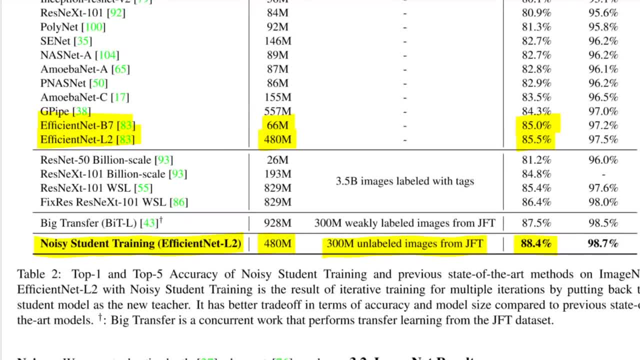 that you have laying around, But the all the information about all the label information comes from the ImageNet data set and comes from this efficient net B seven teacher model. So that's basically you can. it's a testament that out of this, out of this 85, you can make this. 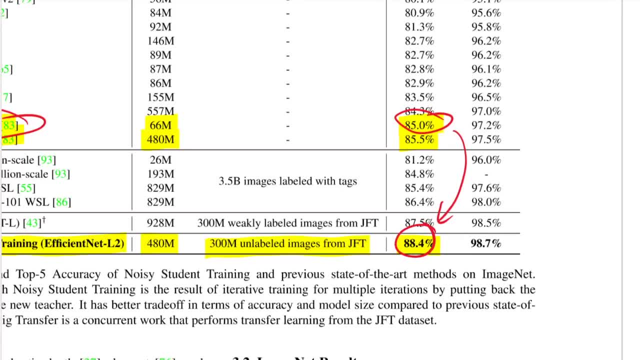 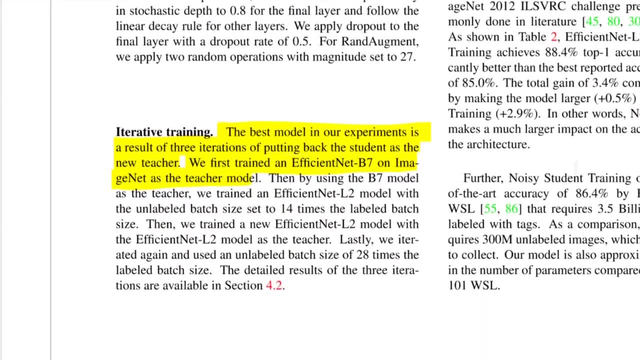 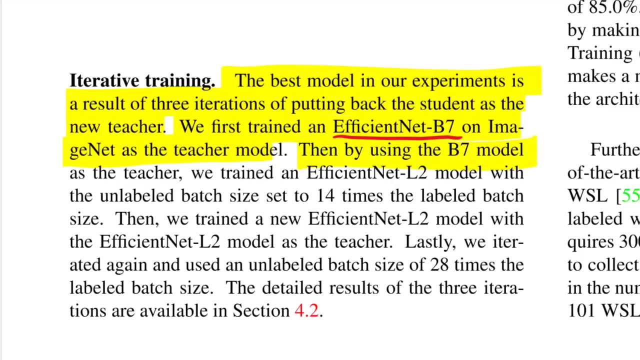 88.. Just by smart, Partly using the information that the model, that this model has learned about the data and transferring it to new data So they train an efficient net. B seven- that's the small model as a teacher model. Then by using the B seven model as the teacher, we trained an efficient net. 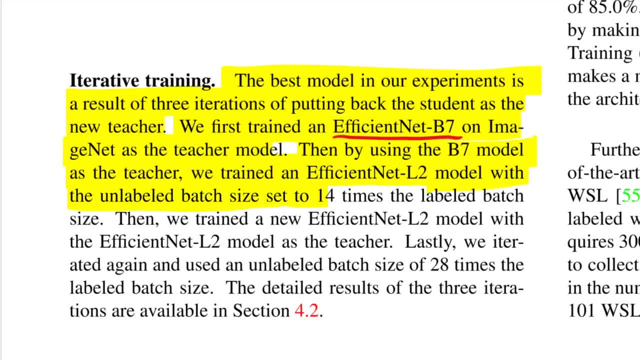 L two model with the unlabeled batch size set to 14 times the labeled batch size, And they stress that it's important that you up the batch size. That's another thing that makes the model more efficient, which is that you can actually if you want to. they just had to. 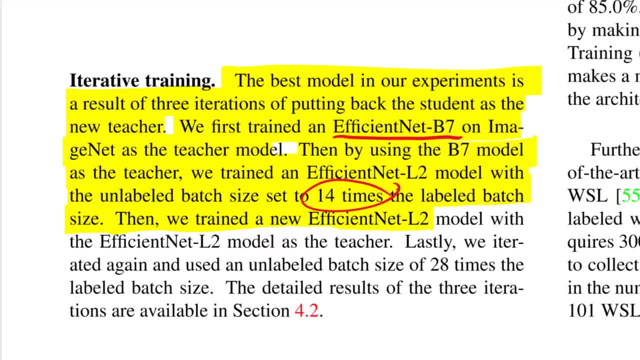 train a new efficient net So you can up the batch size And you can actually learn more than the teacher. then we trained a new efficient net. So, by the way, these this 14 times it's also it can be done, because now you have more data right, So you can also up the batch size. Then we trained a 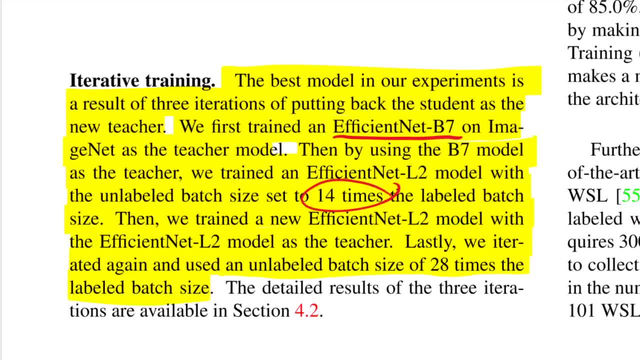 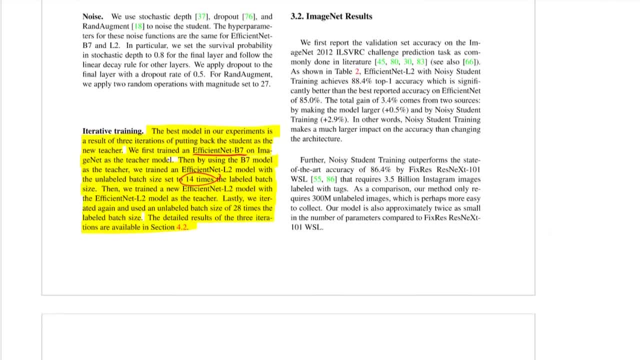 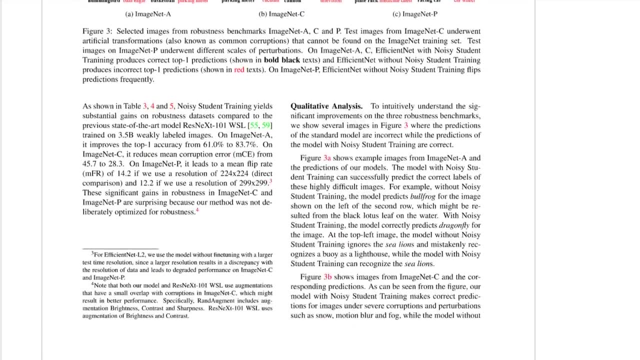 new efficient net L two model, with the efficient net L two model as the teacher. Lastly, we iterated, and so on. Okay, so you can see that it's a fairly complicated procedure, but you can gain and gain and gain by simply up upping the, by simply upping the or iterating on this procedure, And I think 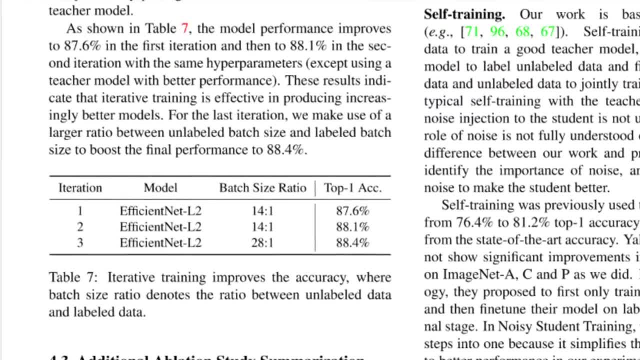 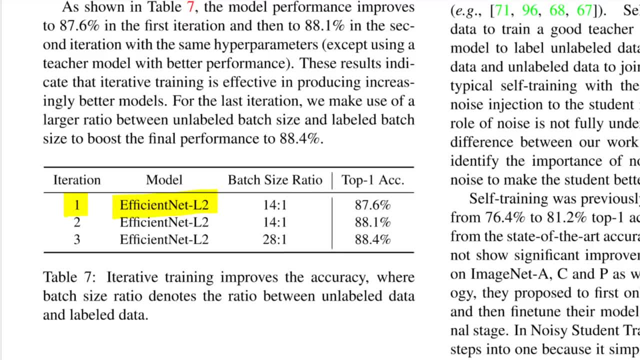 they have it somewhere here. Yes, So, as you can see, if iteration one, you train the efficient, net l two, you start it with the b. seven, you train the efficient at a two with a batch size 14 times larger and you gain significantly. right, this gains about 2% over the original. 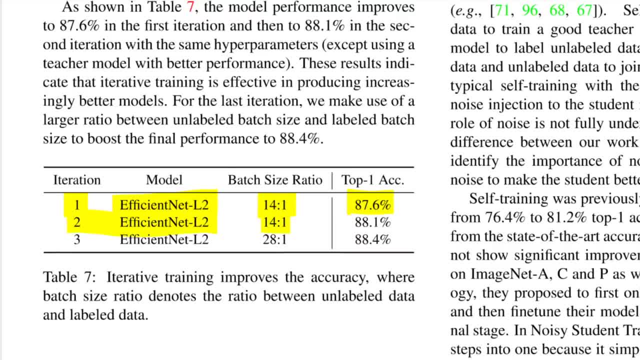 efficient net. then you iterate again with the same batch size and you get like a 5.5% improvement. and you iterate again with an even larger batch size and you get a point 3% improvement. So there's diminishing returns But still you can see that. you know the. 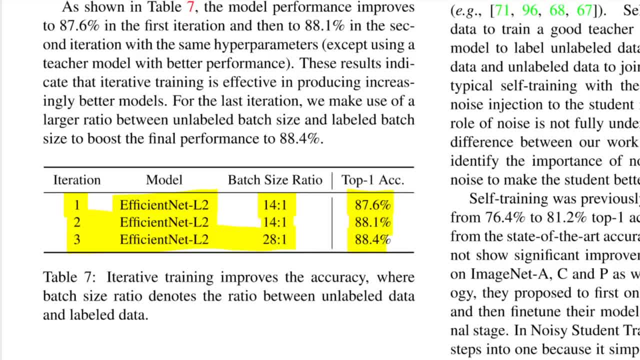 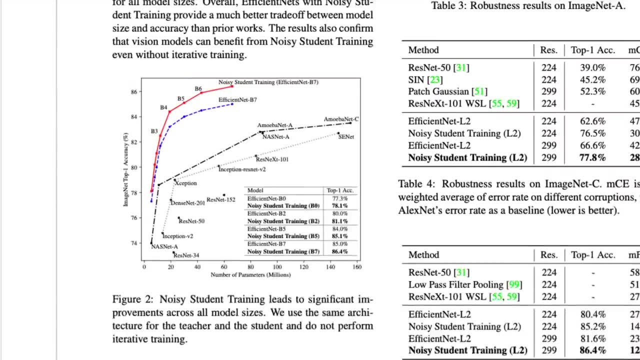 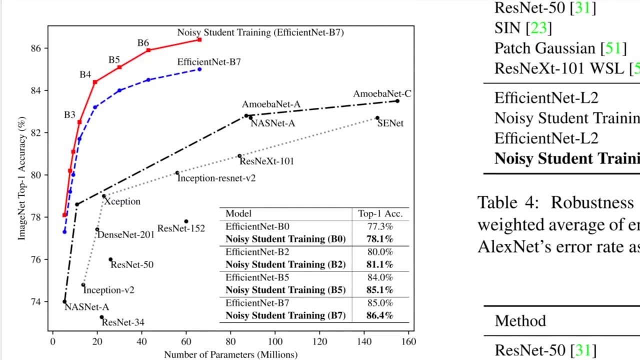 more with the introduction of noise, with the introduction of the larger model, with the introduction of the larger batch size. these are all things that help the student basically become better than the teacher. All right, so they do a bunch of other experiments. So their main comparison is right here, where they say: look if we, if even if we train. 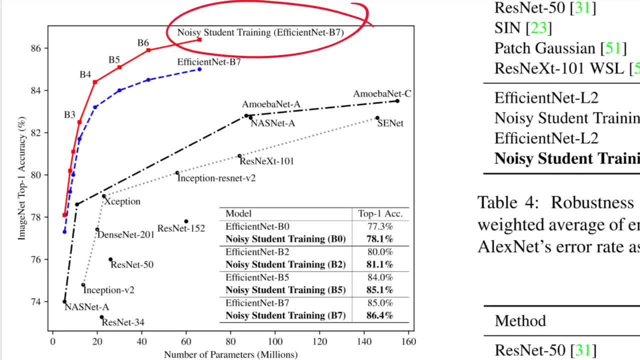 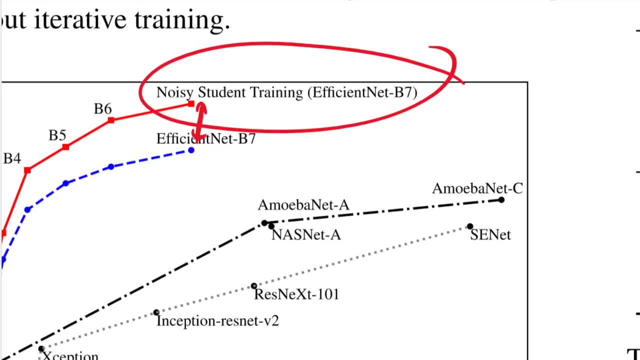 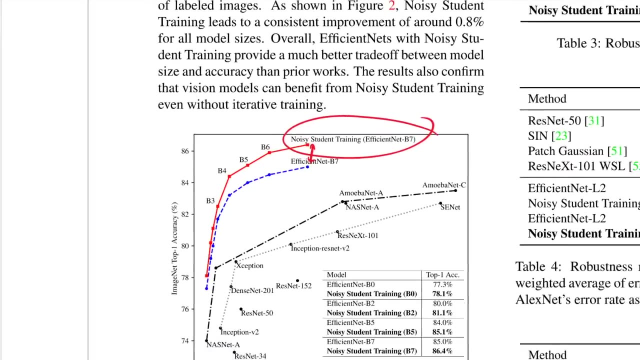 the same model with this noisy student training, we can make, you know, pretty, pretty good, large gains over the model, over the same model where we do not train it with this noisy student training. So this really seems to help, you know, due to the noise, due to the additional data. 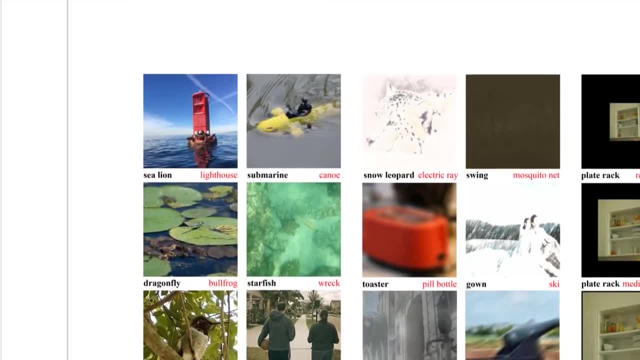 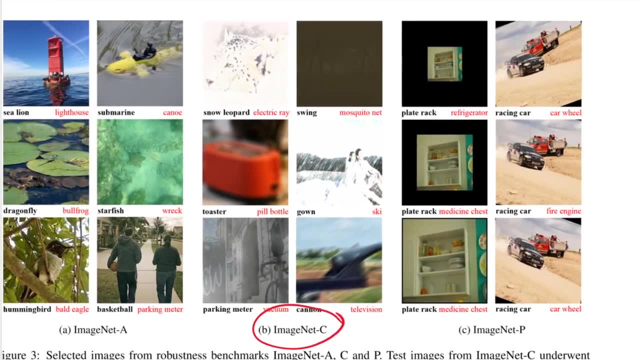 They do a lot of ablation studies, So that's pretty interesting. And they also do these studies on this special ImageNet data set, for example ImageNet C. you can see that there are quite a bit of distortions right here. I don't even see if you can see it on this video, But this is a 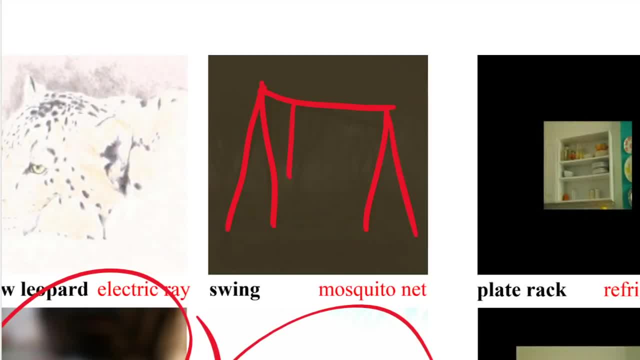 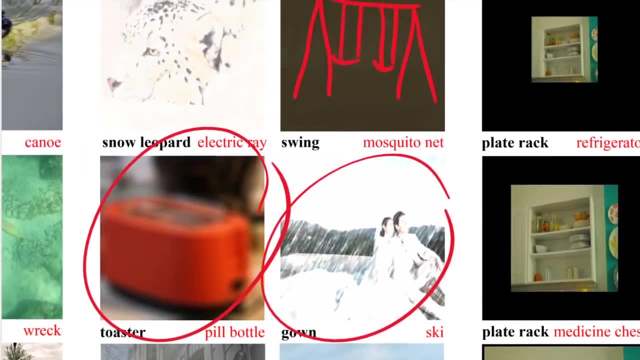 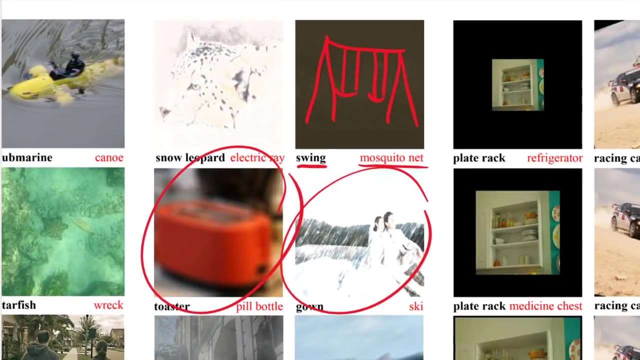 swing. So the swing right here is like something like this, But you almost can't see it. And you see that the bold on the left is always the prediction of their model, while the thing on the right is the prediction of the original model. So this model, they claim, is significantly more. 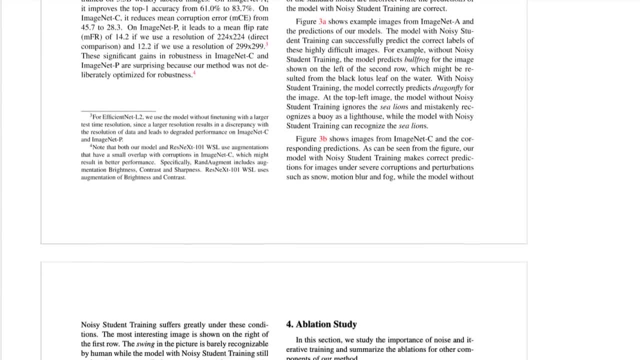 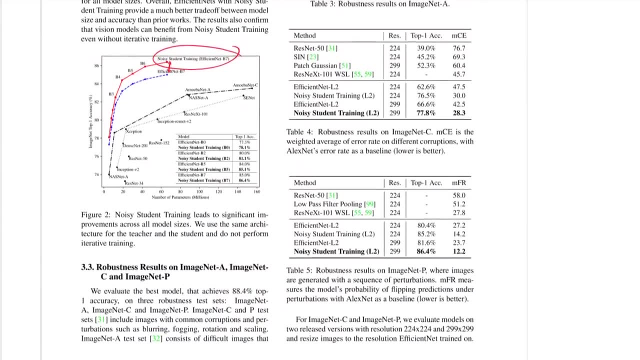 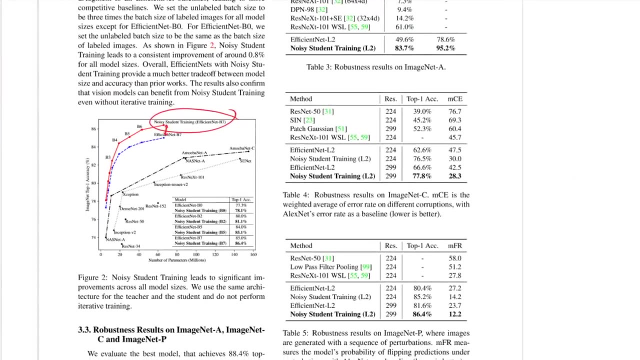 robust to these kinds of perturbations, And they do an analysis of this where they show- Yes, in fact it is So- I think we've already seen this at the beginning- that the noisy student is significantly more robust to these perturbations, And they also test this to. 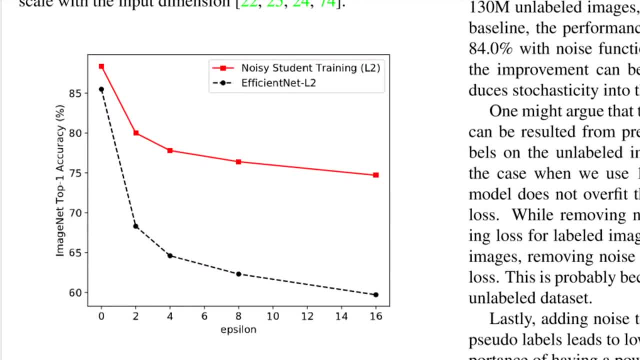 adversarial perturbations. So right here you can see that the original model drops pretty quickly As you increase the epsilon. the epsilon is kind of the strength of the adversarial perturbation And the noisy the model drops very quickly to, you know, fairly low accuracy, while as the noisy, student training drops. 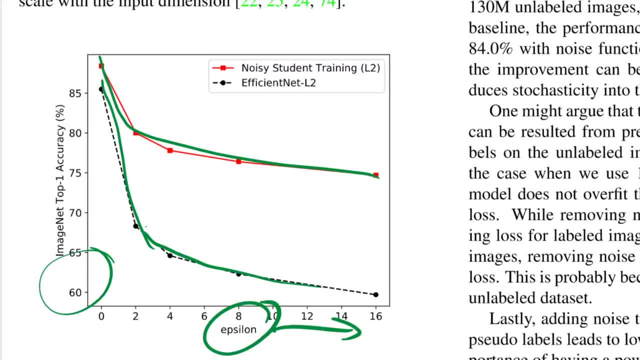 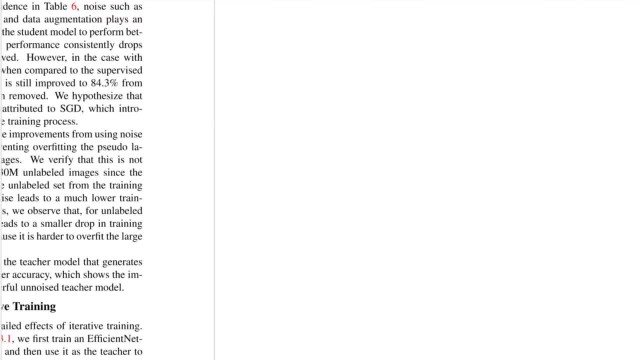 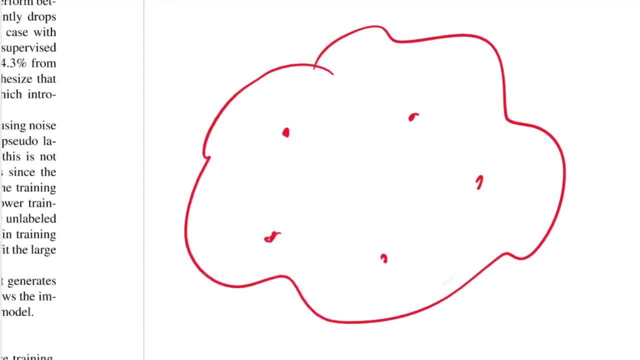 much, much less quickly. Now, this is another testament to the fact that what you do- I think what's happening- is you have your data space right And you have your data points in it. Now, when you do the like- normal data augmentation- what you'll do, is you not? 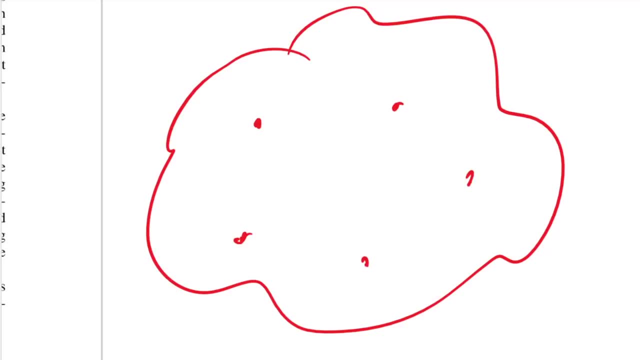 only force the model to predict those points correctly, but you'll sort of make a bit of a cloud around them And you force the model to predict that cloud correctly. Now, if you introduce more data and you do even more noise, what you do is you'll make these clouds kind of larger. 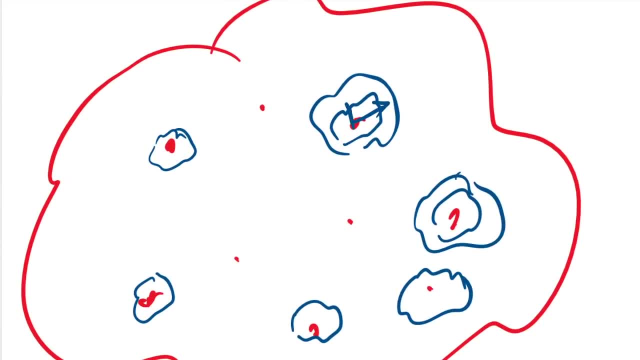 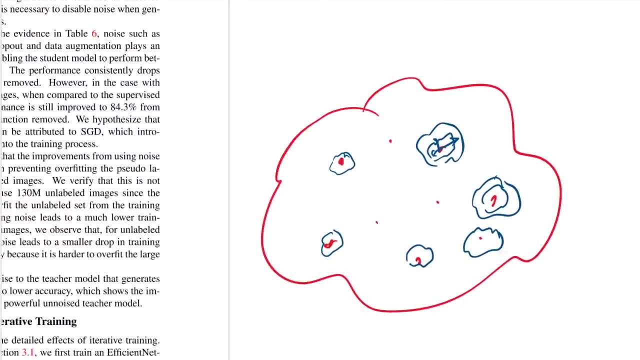 And that means the model is more robust to any sort of perturbations in these clouds right And and that means it's probably also going to be more robust to adversarial perturbations. So that's sort of how you can think of this, this introduction of noise to make it more. 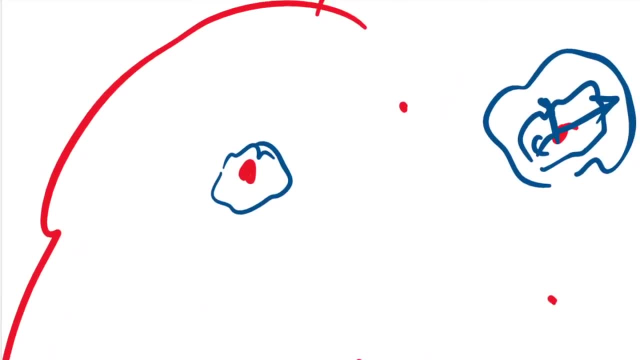 generalizable. How does this generalize better? So, if you think of this data point right here, if I'm looking to generalize, that means you know I have this IID data set, So probably my test data is going to be related to the training data, So I might get a data point. that's fairly. 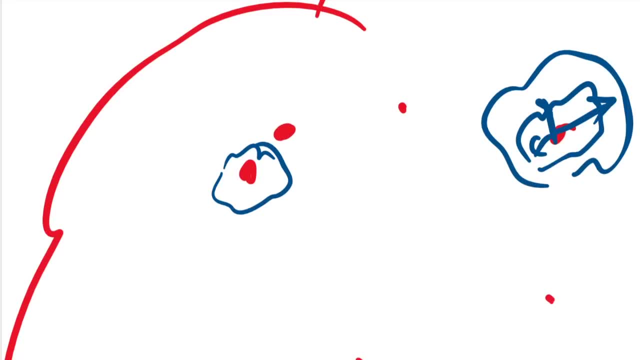 close To that data point And generalizing means I classified correctly. Now, if this cloud is very small like it is here, my decision boundary could be like here: right, And even though the test test data set is fairly close to the original training data point, it's it won't. it will be. 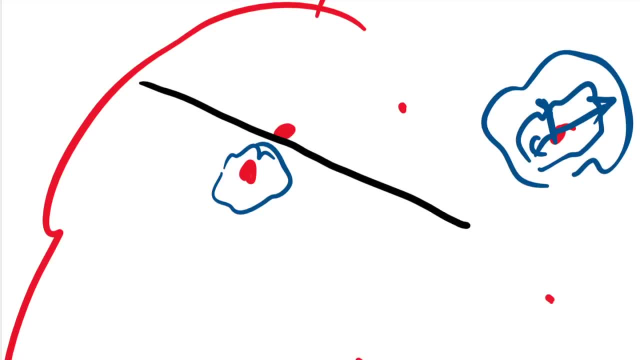 classified incorrectly. However, if my original cloud during training is larger, you can see. if I train a model, it can maybe put the decision boundary here. So I'm going to get a data point here And then my test data point will be included in on that same side. So that's kind of the idea. 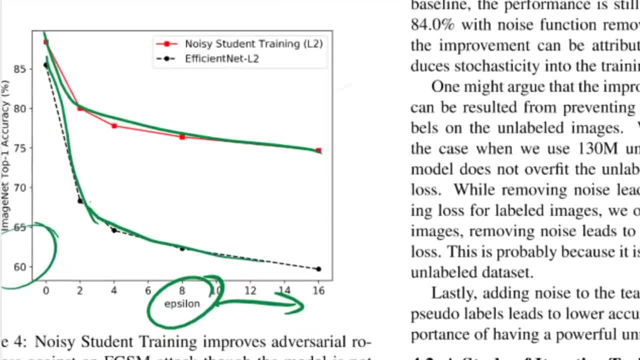 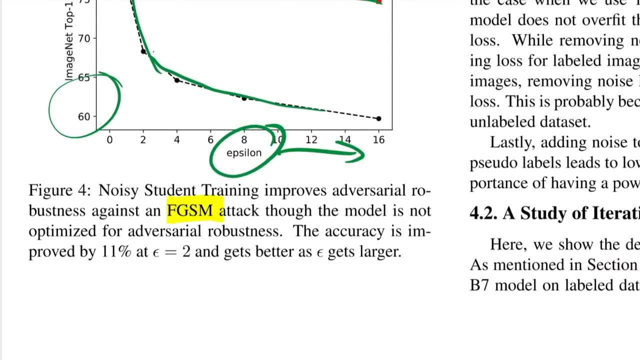 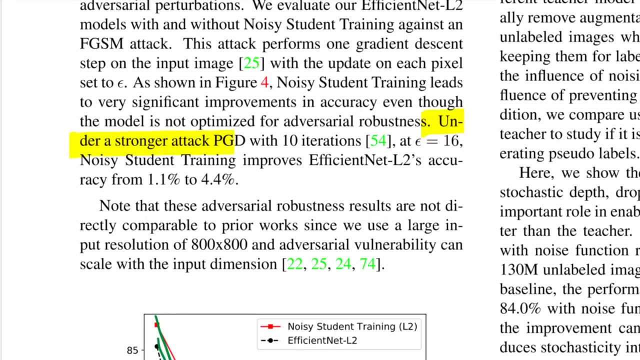 behind generalizing better. of course that's a vast simplification. And also to say that this here is an FGS m attack, So this is kind of the weakest attack in the adversarial perturbation spectrum. They do say under a stronger attack, PGD, which is a fairly strong attack with 10 iterations. 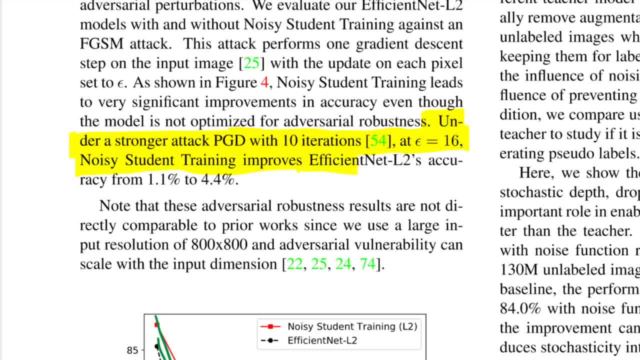 at epsilon equals seven and it's a fairly strong attack with 10 iterations at epsilon equals seven. So this is kind of the idea behind generalizing better. Of course that's a vast simplification And cost 16 noisy student training. improves efficient net l2's accuracy from 1.1 percent to 4.4 percent. 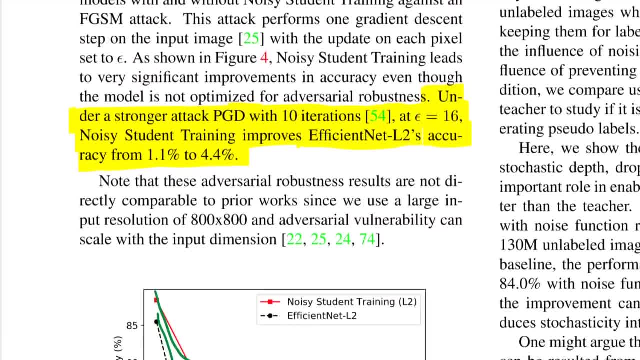 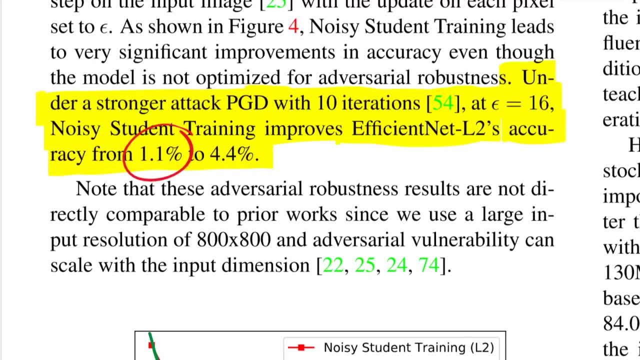 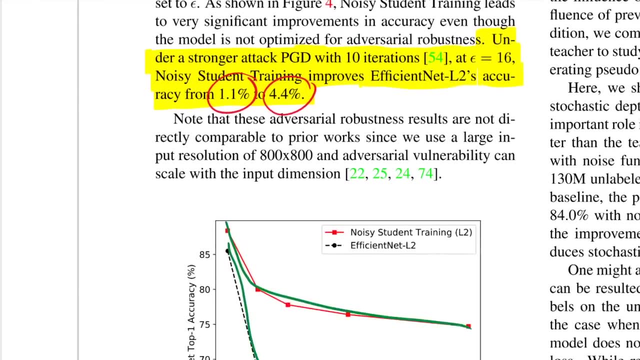 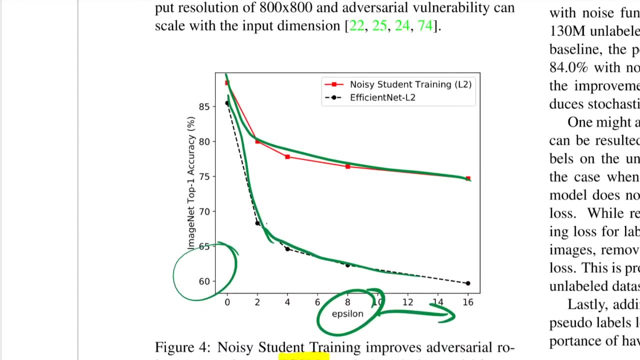 now this, um, like you know, 1.1 percent really means the model is almost like dead. um, this is lower, this is like random performance, and 4.4 percent is still a bit above random performance. but, um, yeah, you could probably. you could probably get there by simply using any sort of noise in. 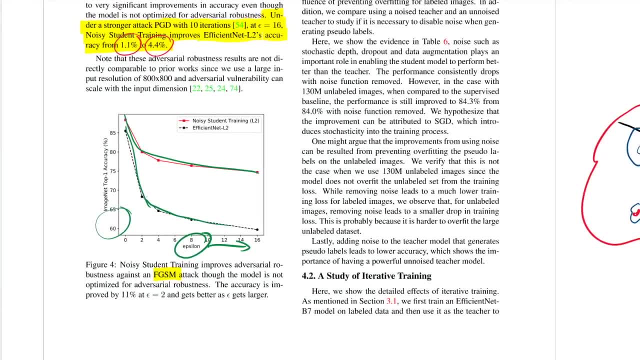 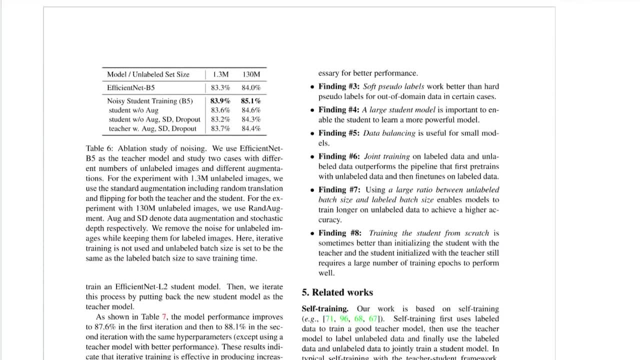 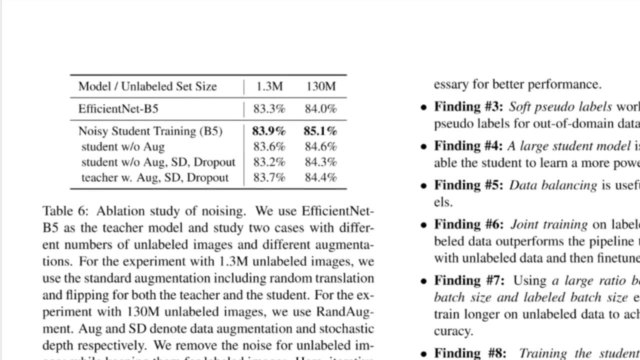 that case, but still you can see that it is more robust to, especially to natural distortions, and therefore it generalizes better. as i said, they do quite a bit of drop- uh sorry, not drop out ablation studies- to figure out where exactly, um, the performance comes from. 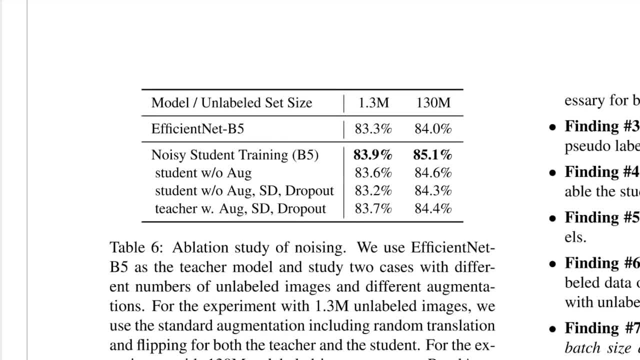 and the answer is it pretty much comes from all the things that they've described. so here you can see um, the in the effect of that extra data set and you can see pretty much, with that extra data set, all the, all the situations improve. here you can see what do you, what is happening when you do. 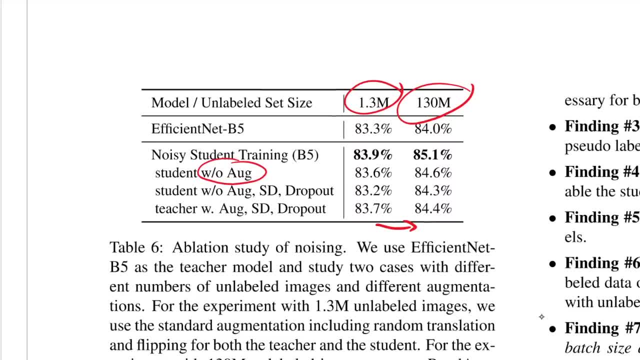 not augment the student. uh, when you do not data augment, you can immediately see that the accuracy drops. and then, when you do not augment and also don't use these model noises, then the performance drops again. and lastly, when you use the teacher, but you noise the teacher, you can see also here the performance is dropping from the. 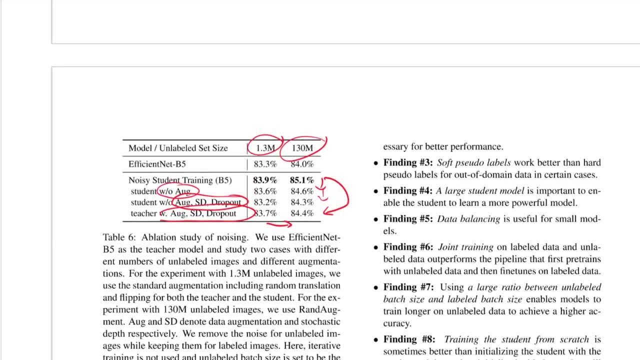 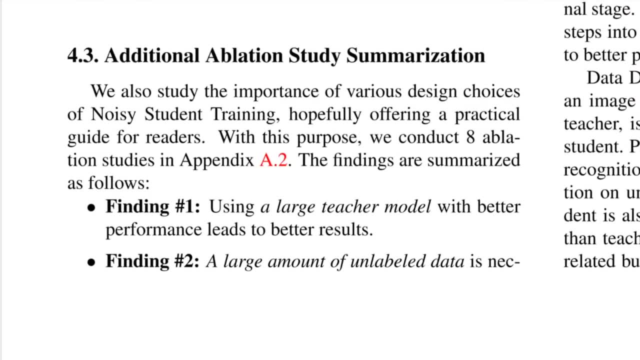 original um quite a bit. so all of these things kind of contribute and they do much more ablations and they have listed their findings here. so using a large teacher model with better performance leads to better result. so you know, as the original model you can see that the performance is dropping. 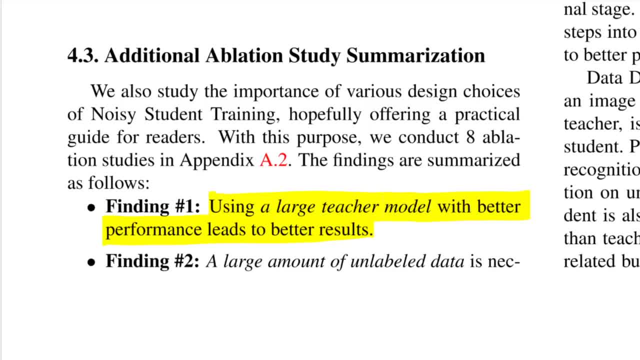 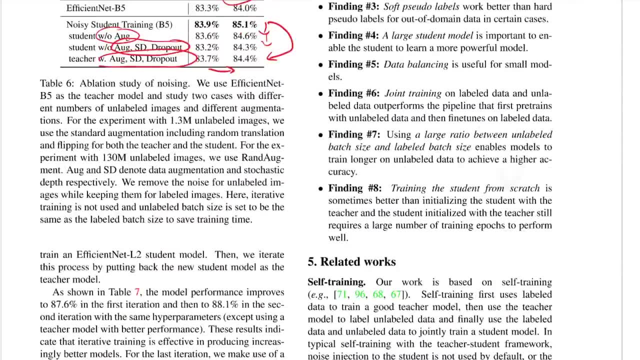 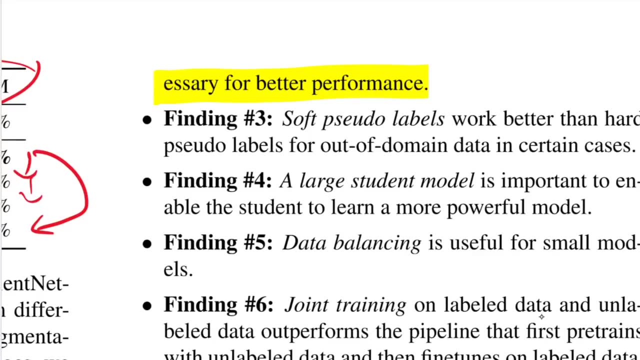 is dropping to the original teacher. you should use, uh, as good as possible, a teacher model you can find. second, a large amount of unlabeled data is necessary for better performance lcd okay. so if you want to do this, you better get a large, large amount of extra data, because that's. 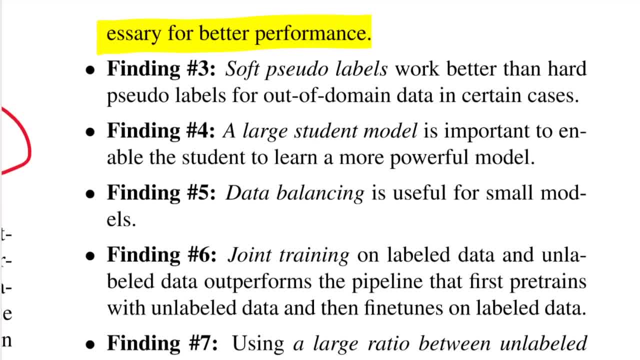 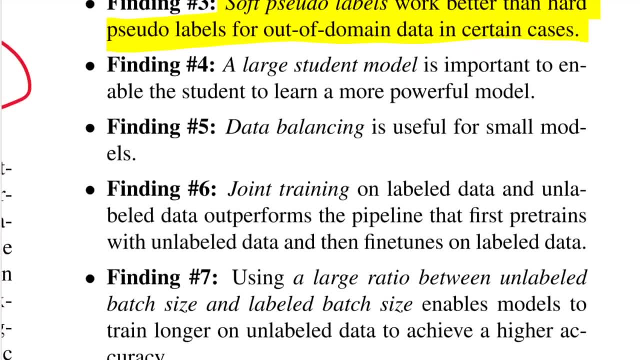 one thing that makes the student perform better. soft sudo labels work better than hard sudo labels for out-of-domain data insert and k? ld, and so do you need more un-labeled models to change performance, cama in certain cases. Fourth, a large student model is important to enable the student to learn a 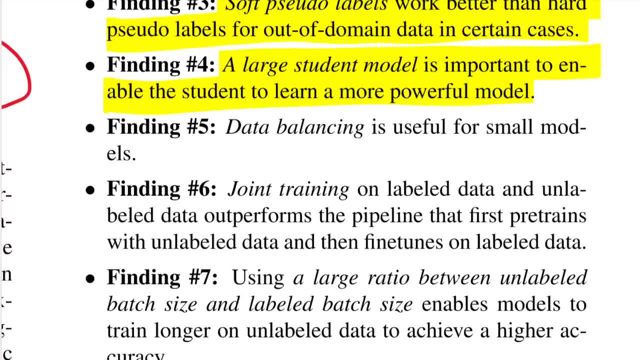 more powerful model. Okay, so, because usually this knowledge distillation is what it. this is usually called knowledge distillation if you use a teacher model to train a student model, and it is often used when the student model is smaller than the teacher. because you want to kind. 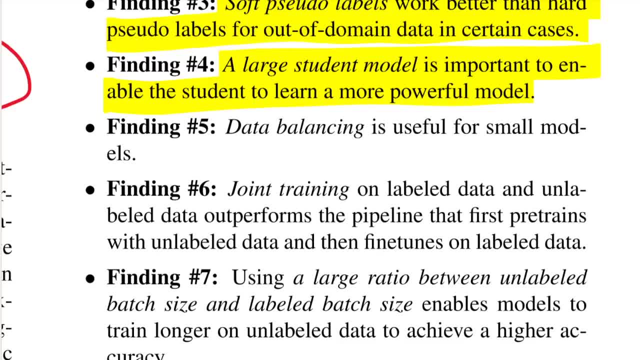 of become more efficient to you from. so the teacher is large, you'll make the student small And you usually sacrifice some accuracy. And here they say: if you want to gain some accuracy you need a large student model, it can't be like a small one. 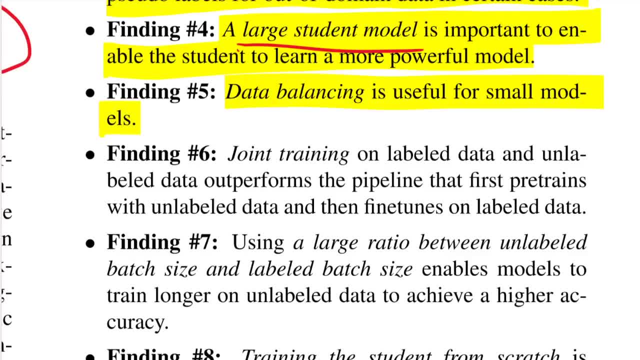 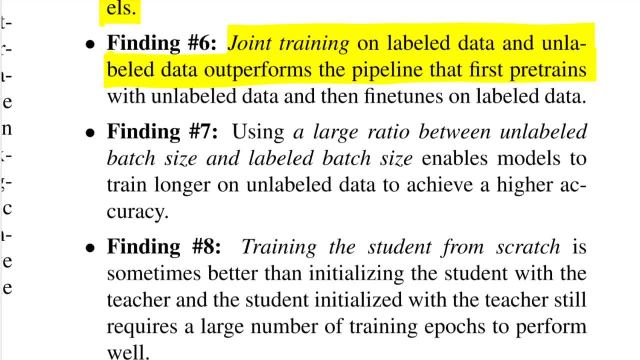 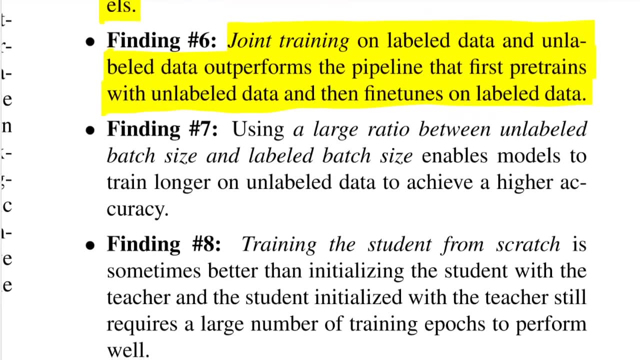 Number five: data balancing is useful for small models. Number six: joint training on labeled data and unlabeled data outperforms the pipeline that first pre trains with unlabeled data And then fine tunes on labeled data. So this is in contrast to like what people have done before in 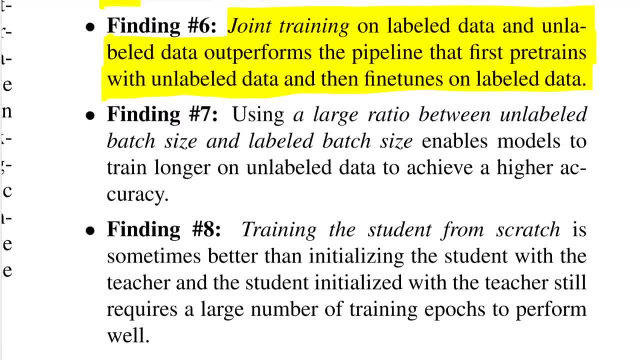 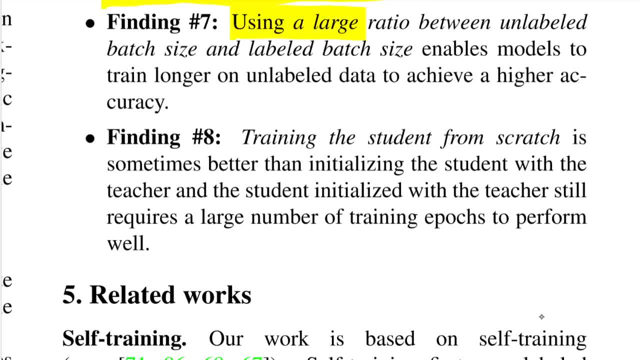 the self supervised learning and so on, where it's always kind of pre training, then fine tuning or in the in the transfer learning setting. Seven: using a large ratio between unlabeled batch size and label batch size enables models to train longer on unlabeled data to it to achieve a higher accuracy. 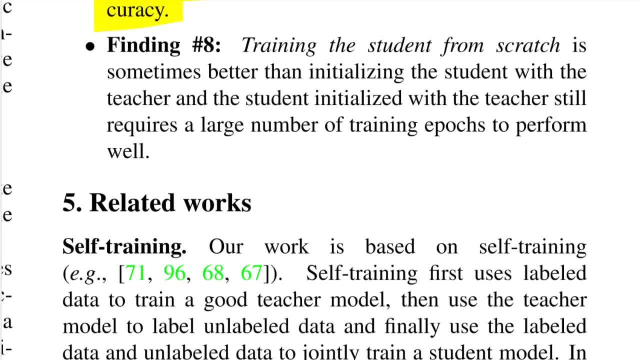 Okay, we've already seen that they have used that. And number eight: training the student from scratch is sometimes better than initializing the student with the teacher, And the student initialized with the teacher still requires a large number of training epochs to perform well. This is fairly interesting because it 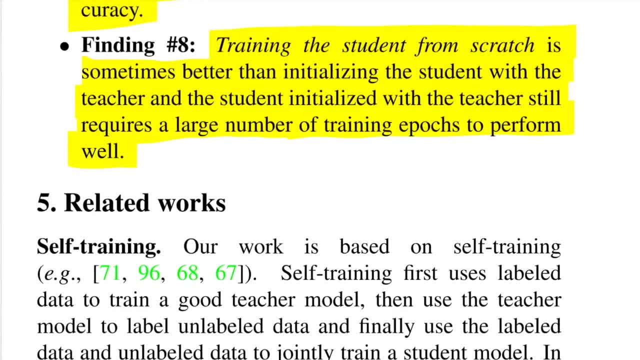 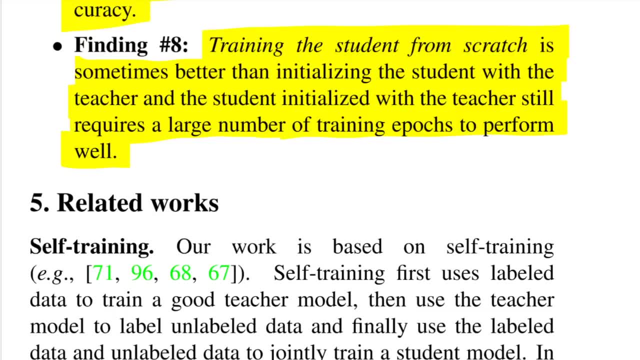 kind of alludes to the fact that the minima in weight space, if so, if this is of course the case, if the student model is the same as the teacher model, so in like iteration two or three or whatnot, It means that you know, in weight space, if we look at you know you might want to start the 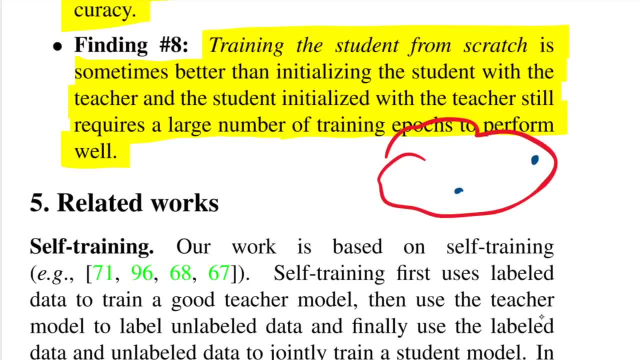 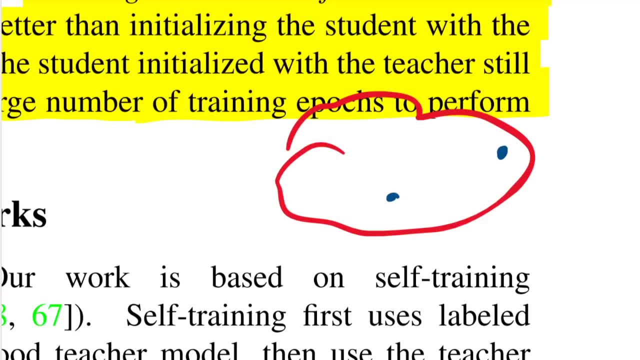 student here and the minimum is right here. And you might want to think that if I learned the same thing, then the minima are fairly close together, right? So the the teachers minima might be here and the student minima might be fairly. 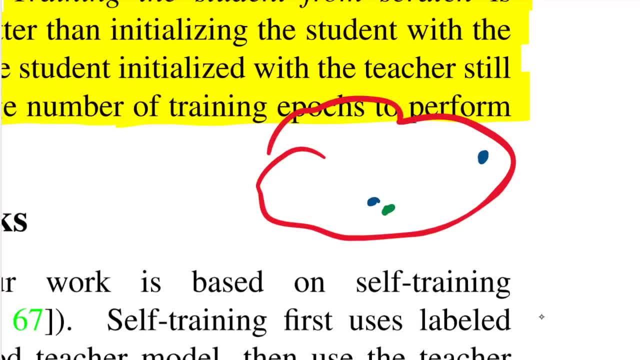 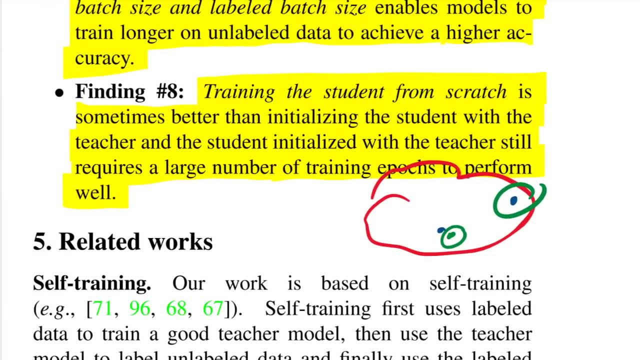 close. So it might be beneficial if I- if I start not over here, but actually start at the teachers minimum. But this doesn't always seem to be the case, And that is a fairly interesting observation, because it kind of means that we're talking about different minima. here we're talking about the 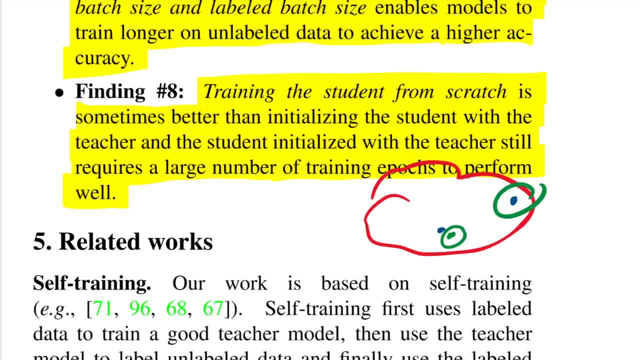 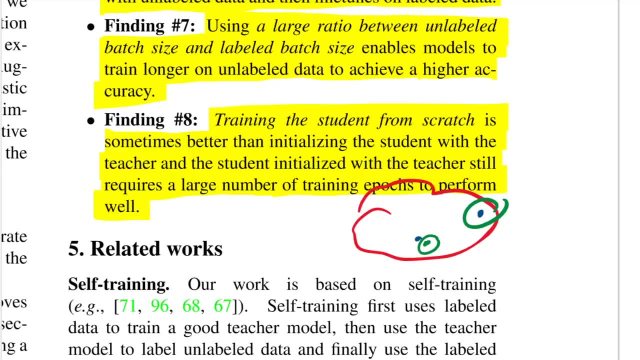 student model learning different things, And that's what we've discussed already. the student model kind of learns to be robust And that's probably a minimum. that's fairly far away in weight space, at least in in a sort of energy landscape, weight space might be the case that. 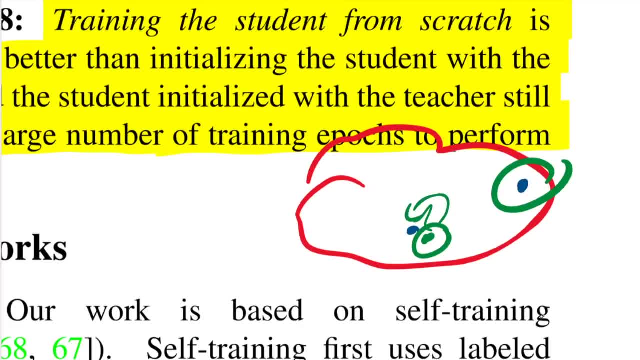 it needs to actually overcome kind of a hill here, even though the minimum might be close. There's lots of research in like how minima are distributed in these weight spaces, which I don't want to go into right here. But it is a fairly interesting observation that it's not. 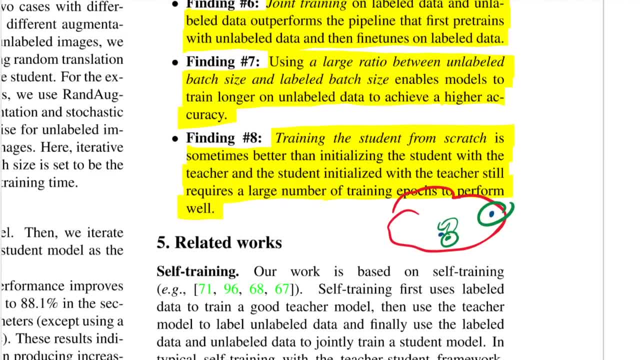 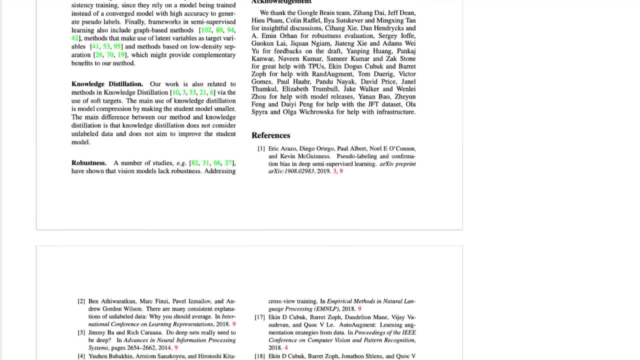 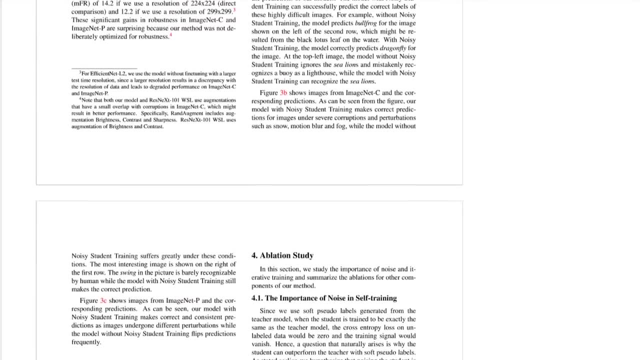 always helpful to initialize the teacher- sorry, the student- at the teacher's optimum. Okay, so this was the paper And you know this is. this is a type of research where I do appreciate kind of the these large labs taking it on because they 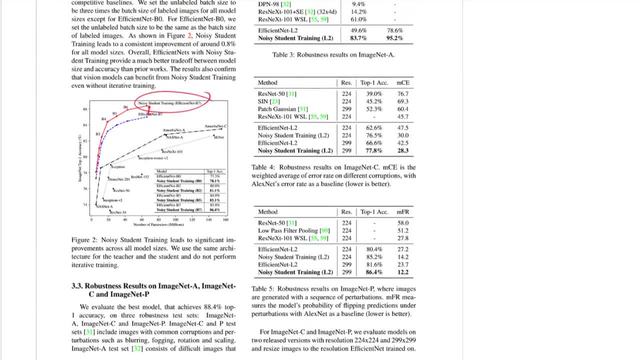 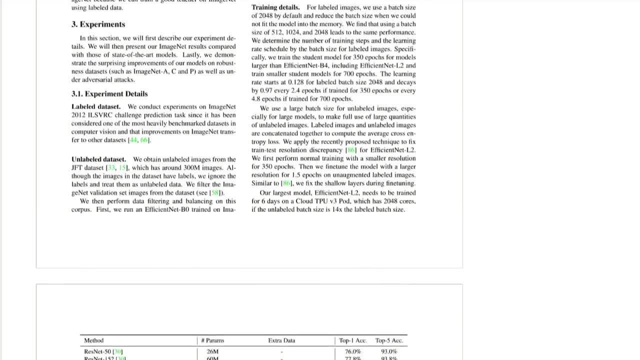 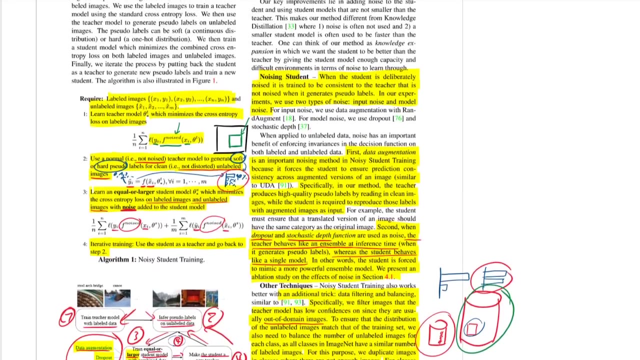 have the resources to do all of these ablations, all of these different models, cross them with these giant data sets and so on which I guess university labs just would not have. And this is a fairly thorough paper really investigating which parts of the pipeline you know do something and 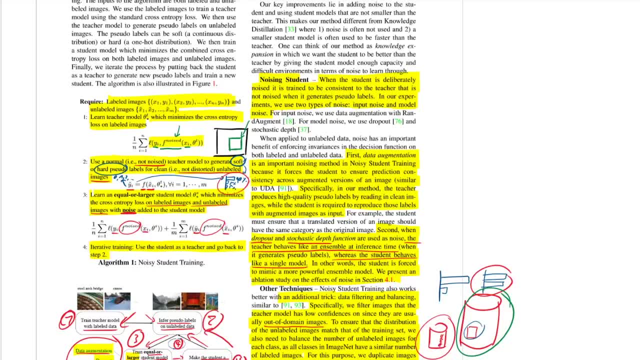 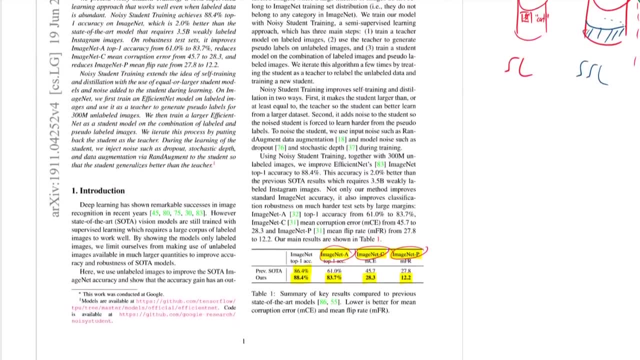 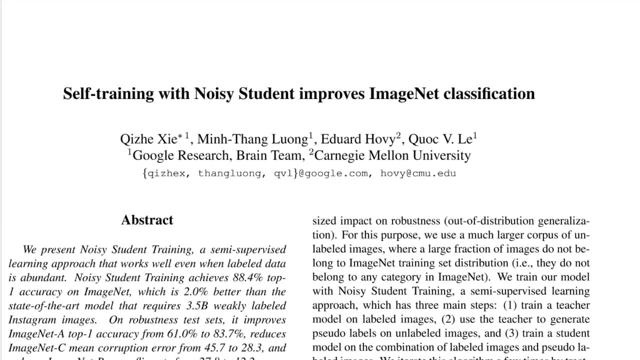 which ones don't, And usually I I'm fairly critical of pipelines that have like 50 billion tricks, because you never know where the improvement exactly is coming from. But you can sort of mitigate that criticism by doing all of these kind of ablations on the different parts.